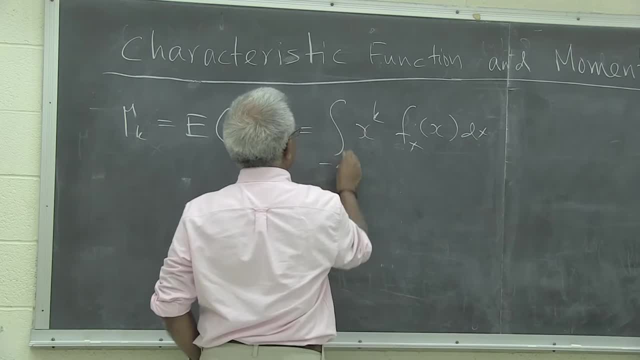 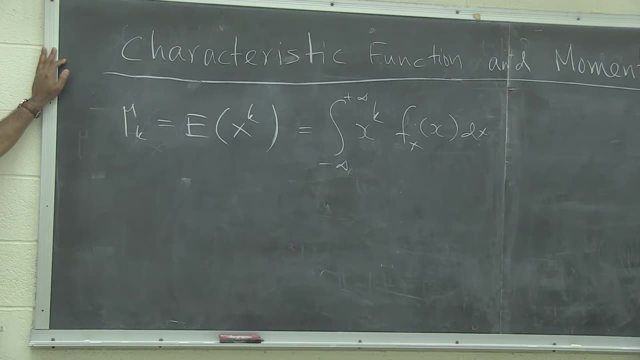 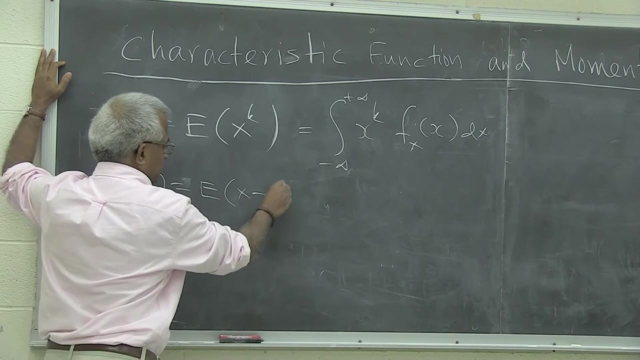 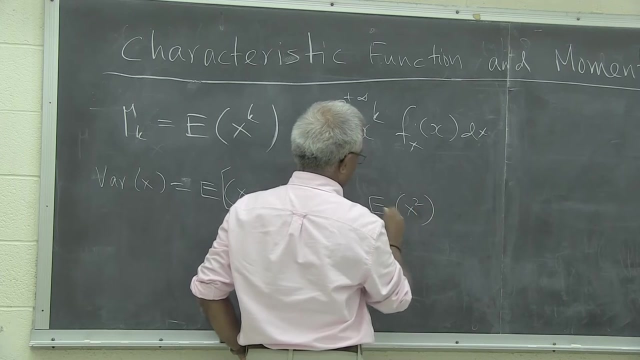 function of x- dx. so you need the first order and second order moment to compute the variance. and so, for example, variance of x is expected value of x square x minus mu, the whole square. but this if you expand you can show it to be expected value of x square minus expected. 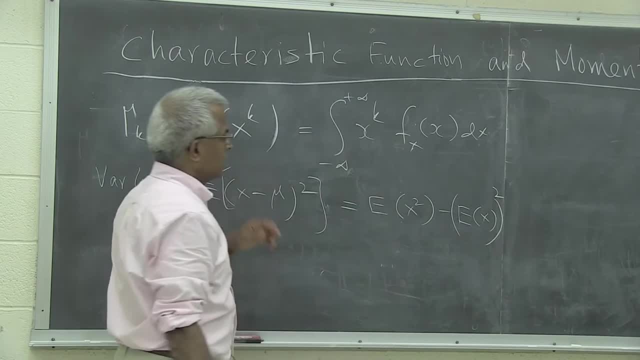 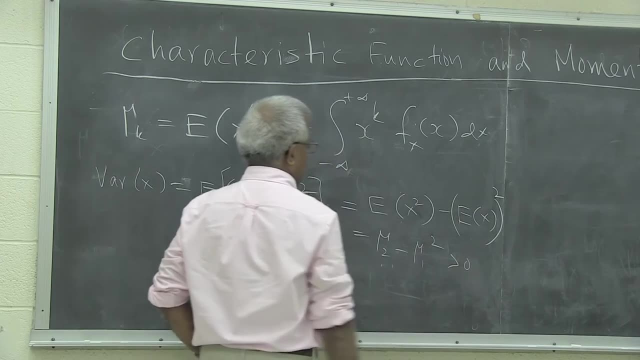 value of x, which is mu the whole square. So you can see the. so this is, if you want, you can this above notation we can write it as mu 2 minus mu 1, square the whole. so these moments are important, but the computing 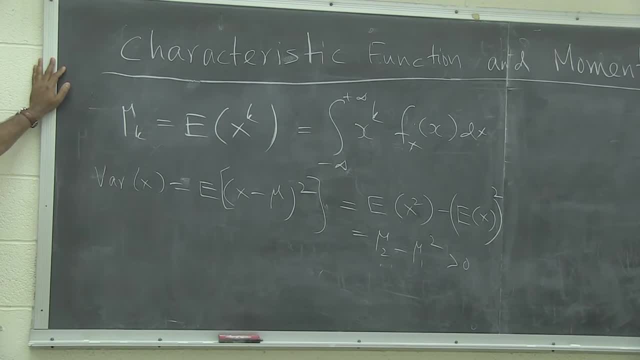 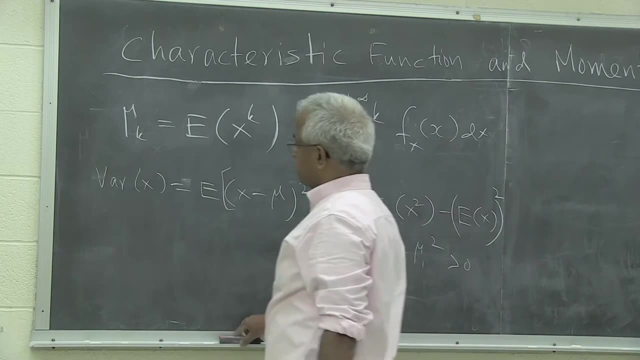 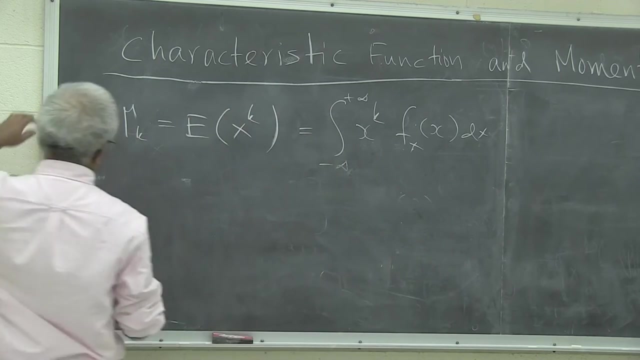 moments directly. sometimes it takes lot of time. so this concept of characteristic function is useful. so let me define what the characteristic function is. then we could do this for for few random variables. so characteristic function of a random variable is defined, as expected. 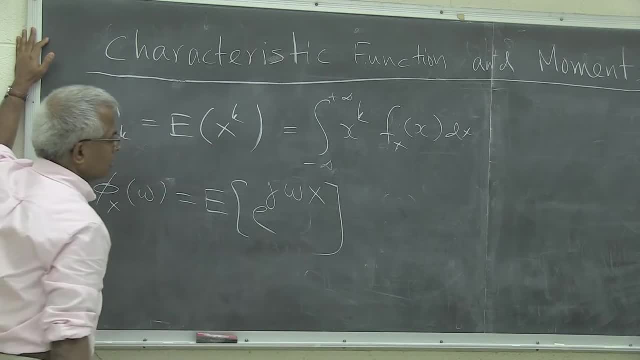 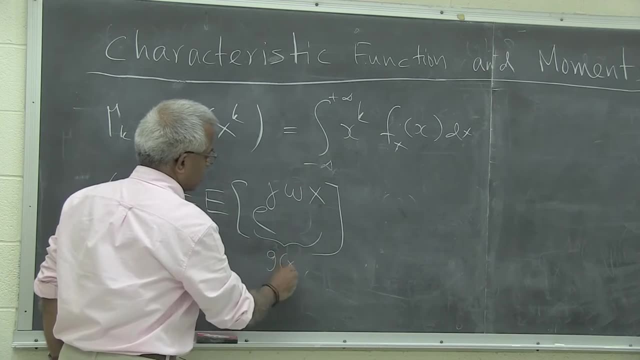 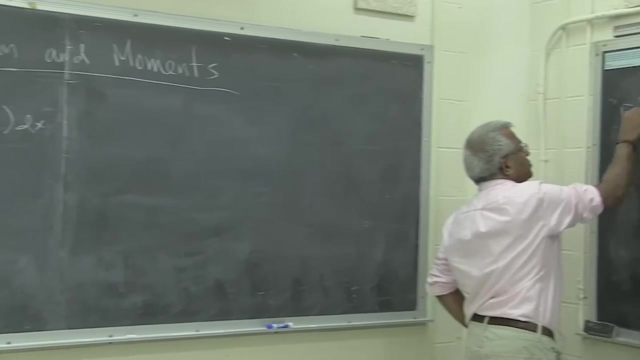 value of E raise to J, omega x. So this is where the random variable is. so this is like one function of a random variable, g of x. so expected value of g of x is here right. expected value of g of x is g x multiplied. 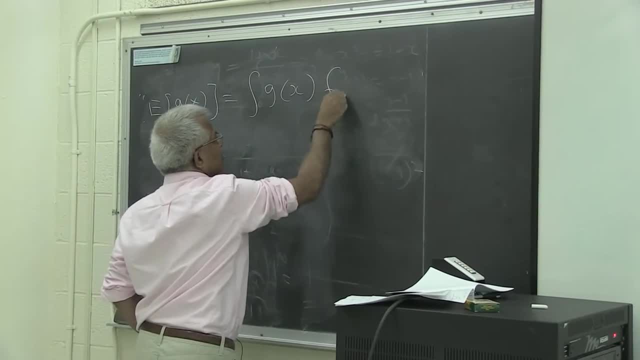 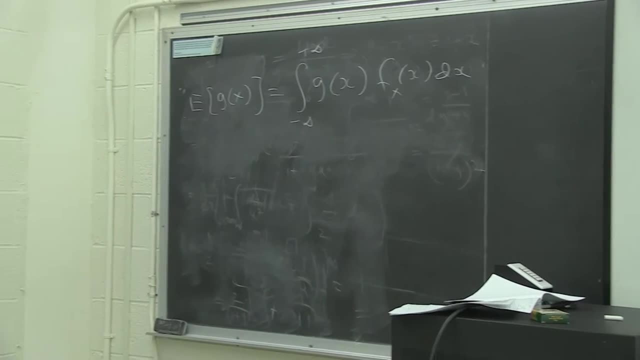 by the density function of x. So x square, I mean x square, this is equal to. so this is like I will write this. so of x, dx, just like here. expected value of x to the power k is the function multiplied. 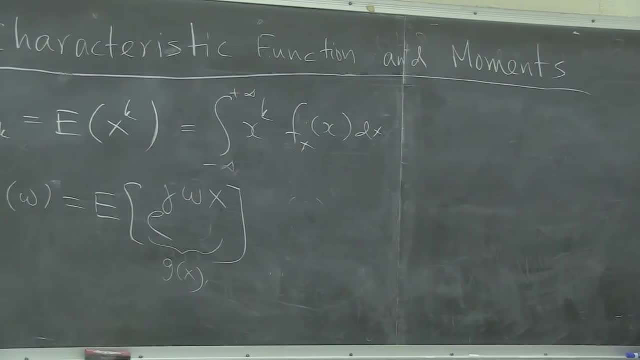 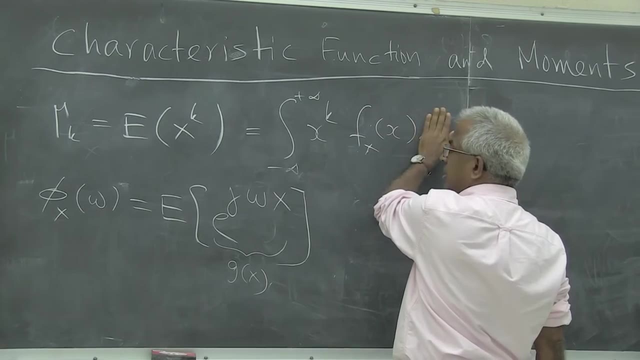 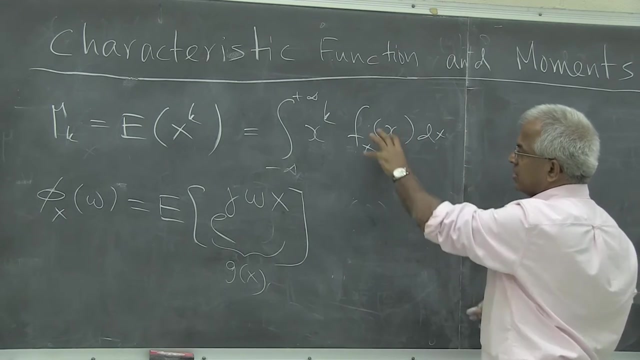 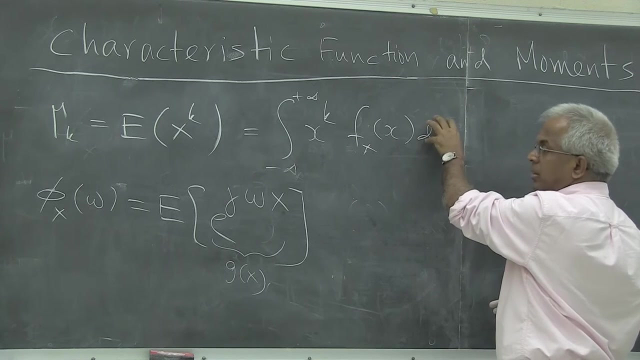 by the density function. so because the argument is you call this to be y, this is y multiplied by fy, dy, but y is of course g of x and fy. we can write it in terms of fxx as fxx multiplied by 1 over dy, by dx multiplied by dy. so dy cancels and the dx comes and you get this. 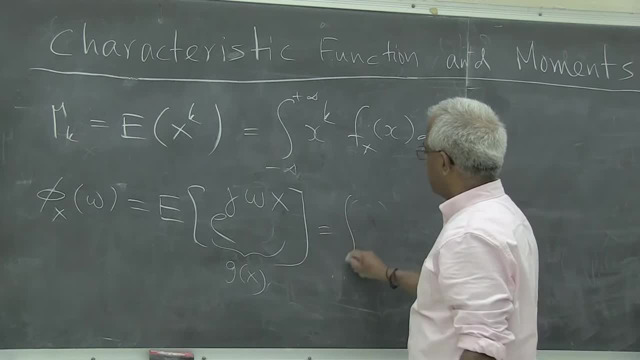 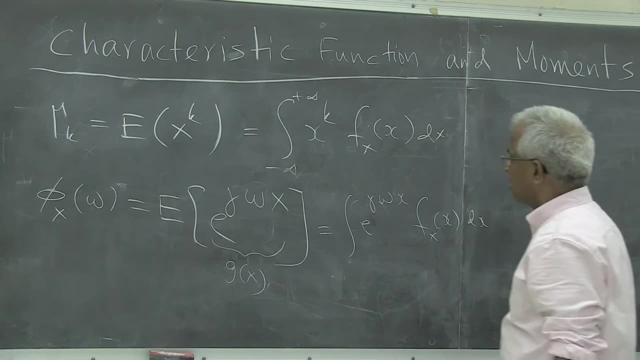 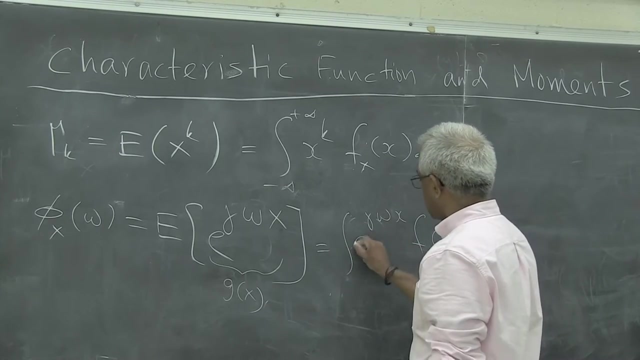 formula. So this is using the same formula. this is e raised to j, omega, x, fxx, dx. so you just need to compute this for various density functions, which we will do in a minute. But let me show you one useful application of this. so if I expand this e raised, so 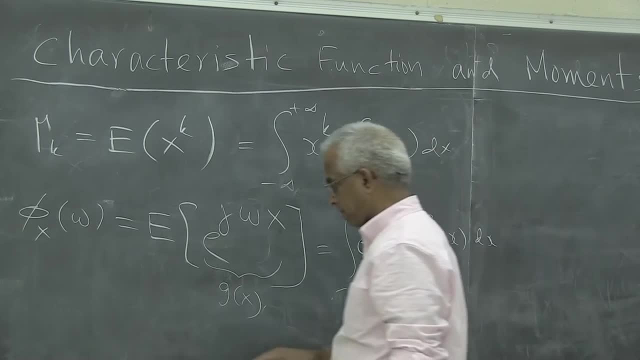 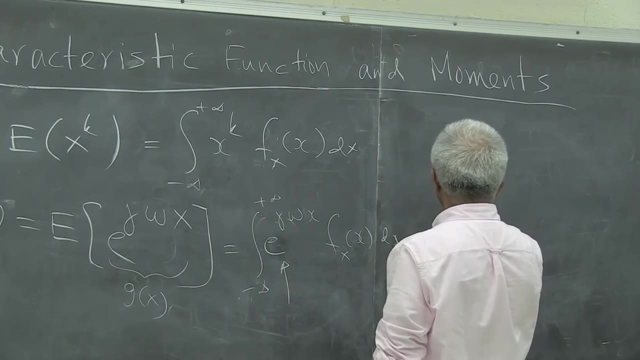 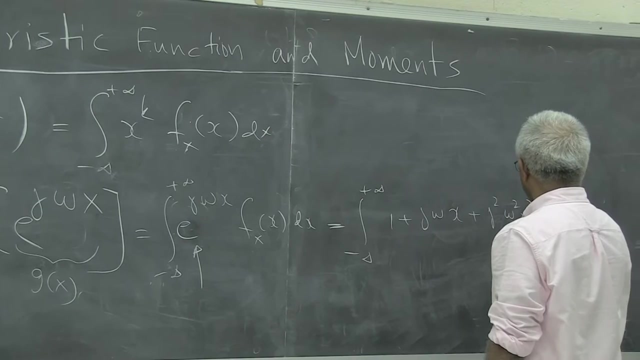 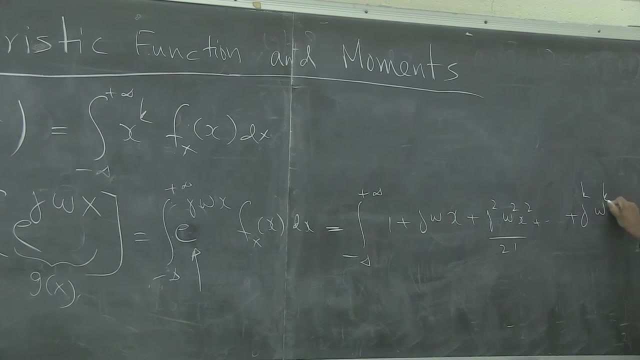 this is from in general, minus infinity to plus infinity. And if I expand this e to the power j, omega x term, that is 1 plus j, omega, x plus j, squared omega, squared x, squared 2, factorial right, etc. j to the power k, omega to the power k, x to the power k over k, factorial, etc. it goes: 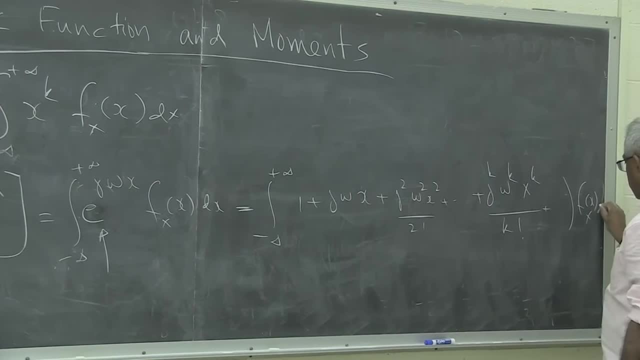 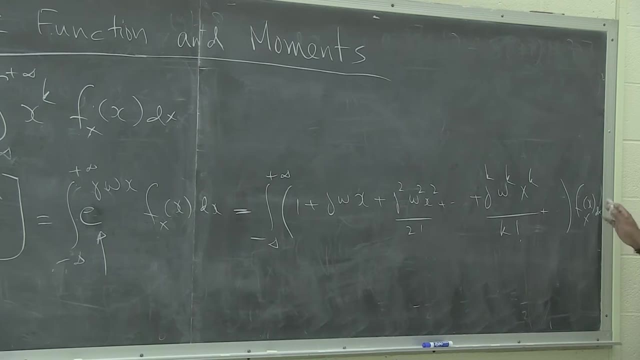 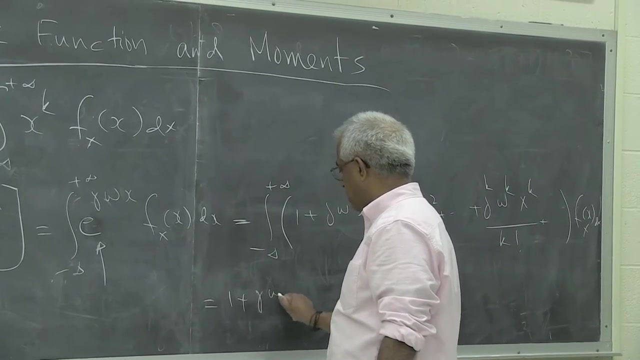 on, multiplied by the density function of x, dx. So this is just the expansion of e raised to j omega x. so notice: the density function multiplies each term, so the first term will be a constant. then you have j omega x multiplied by the density function. 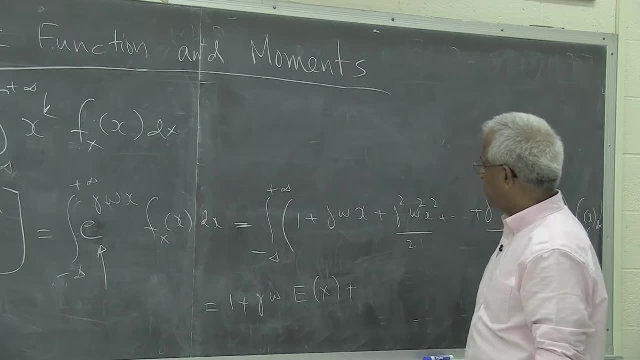 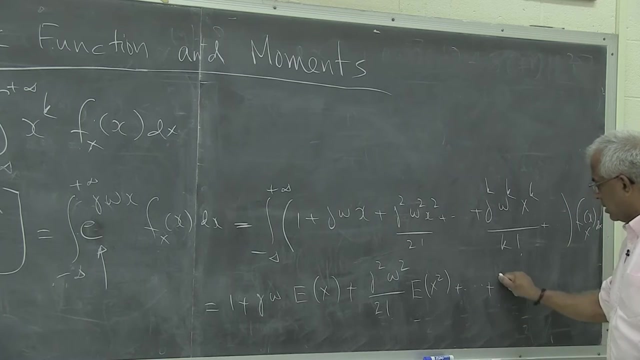 So that's going to be expected value of x plus. the second term is j squared- omega squared over 2 factorial, x squared multiplied by the density function dx. so that's expected value of x squared plus, etc. j to the power, k, omega to the power k over k, factorial. then 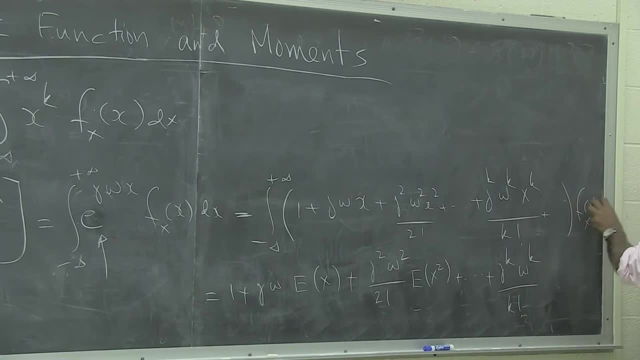 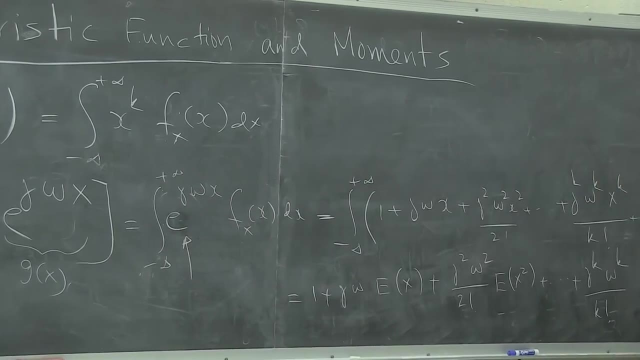 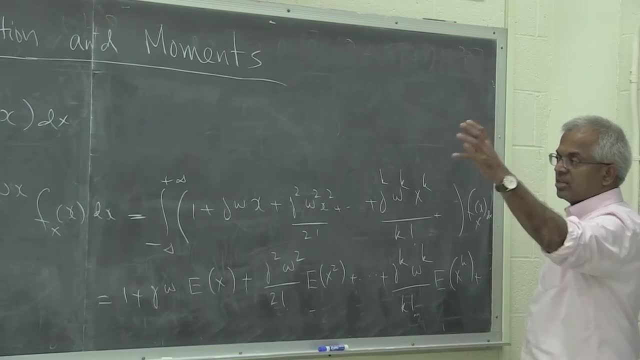 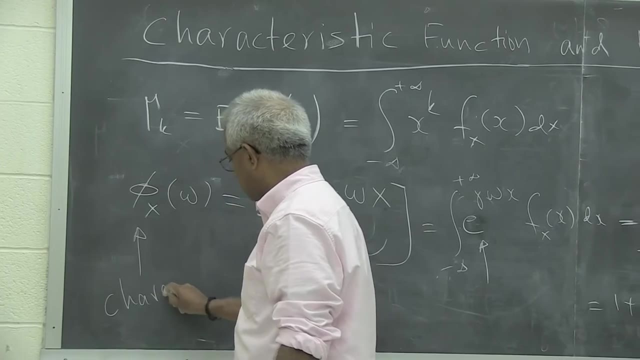 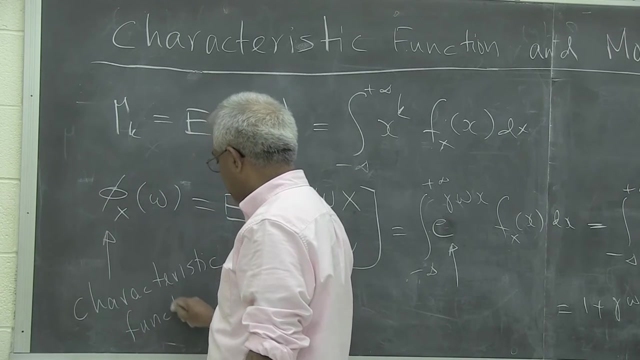 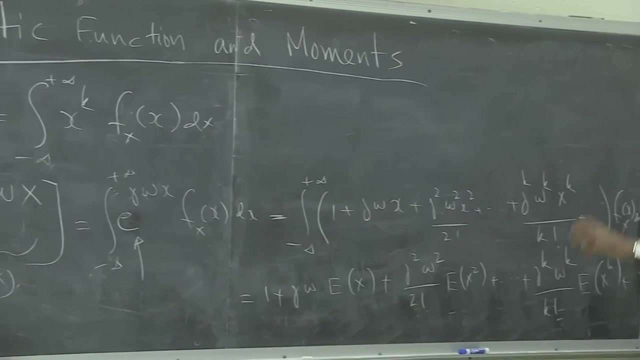 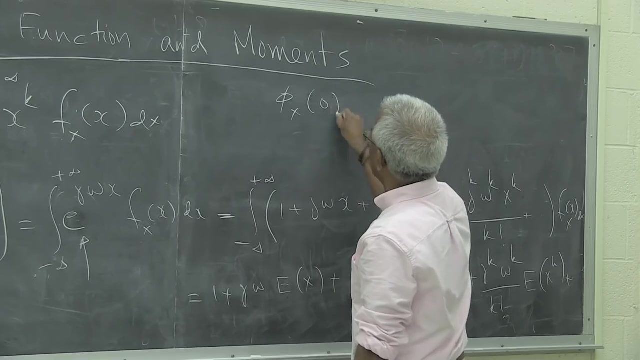 xk plus, etc. So the interesting thing is, this function, which is the characteristic function, has all the moments embedded in it. So how do you? You can compute the moments from the characteristic function, because the answer is right here. So notice that. first of all, you notice that if you put the characteristic function omega 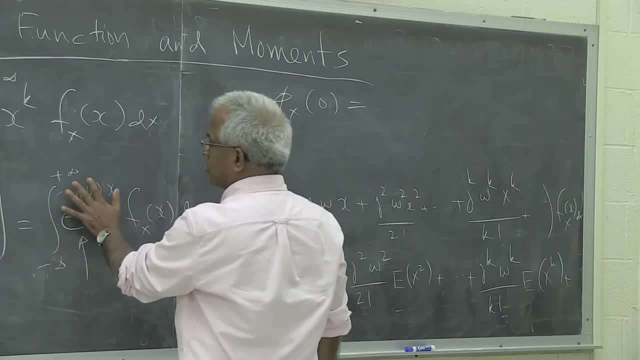 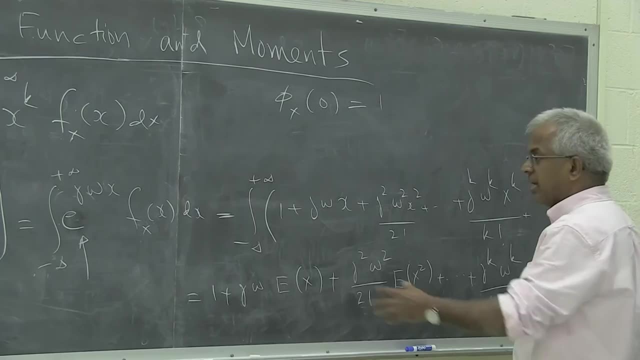 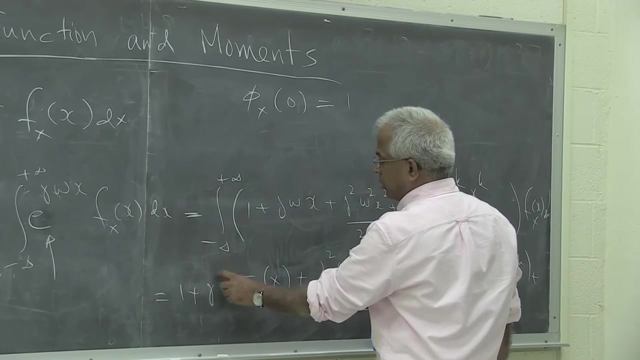 equal to 0,. you can see omega equal to 0, this is 1, that's just the area under the density function. So this is 1, now if you take the derivative of this with respect to omega, you can see here: the derivative is constant here. so the derivative with respect to omega is this: 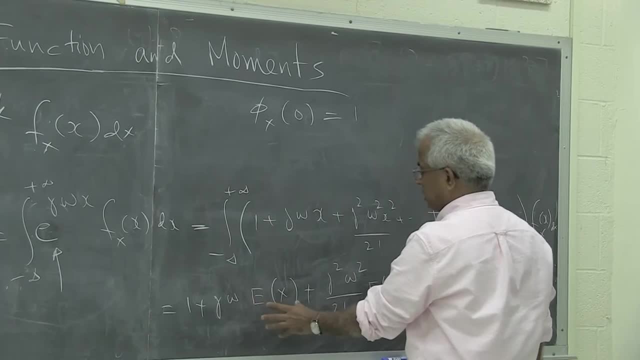 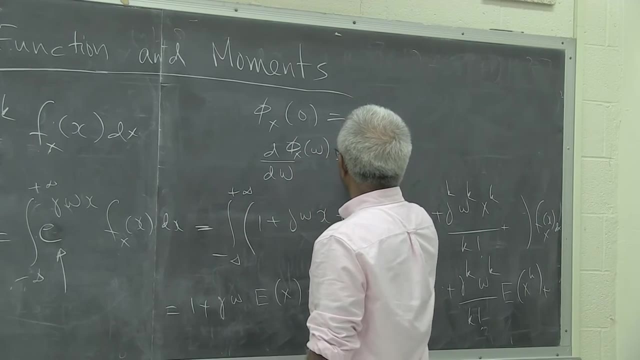 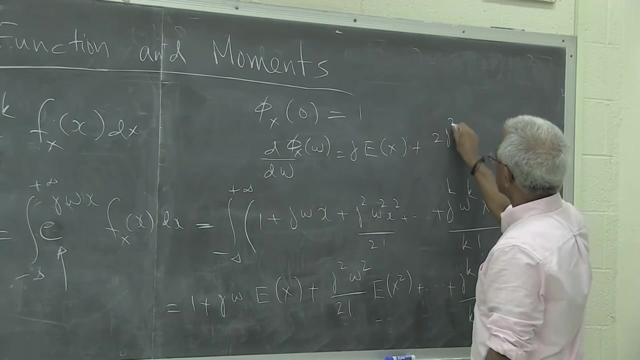 this is all a constant, so just one here. so if you start taking the derivative of characteristic function with respect to omega, you get j multiplied by ex. but if you look at the next term, it is going to be 2 omega 2 j squared omega over 2. factorial expected value of x. 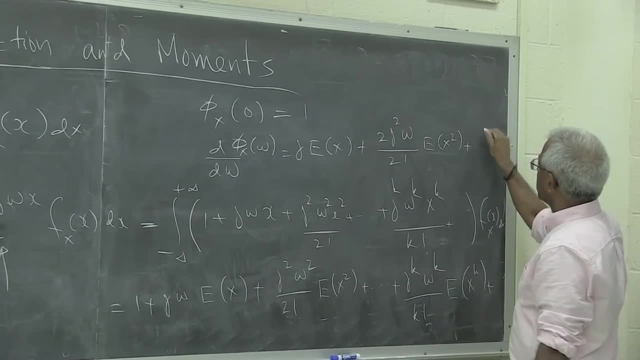 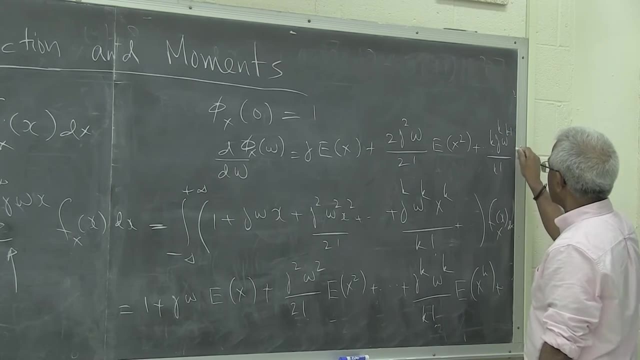 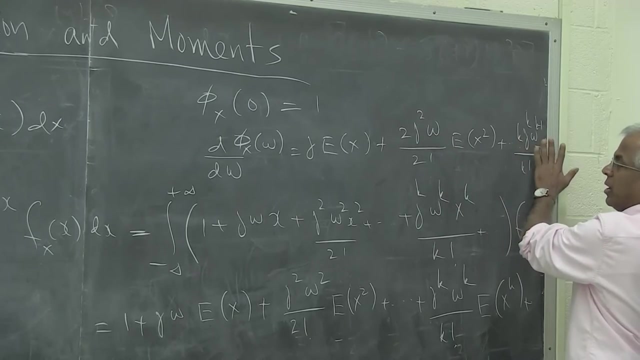 squared and in general from here it will be k: j to the power k, omega to the power k, minus 1 k factorial expected value of x to the power k. Now is an interesting thing: everywhere there is omega here. so if you put omega equal to 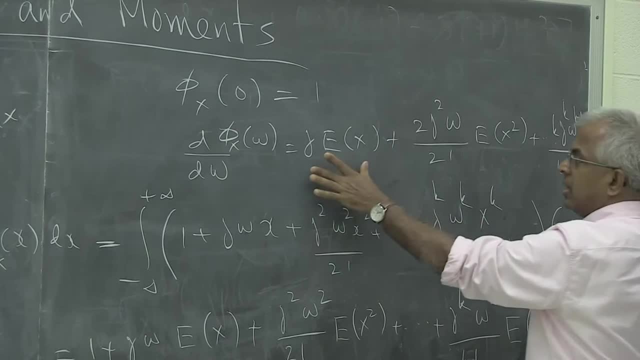 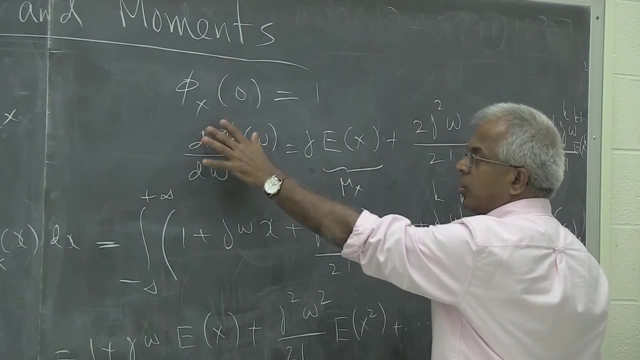 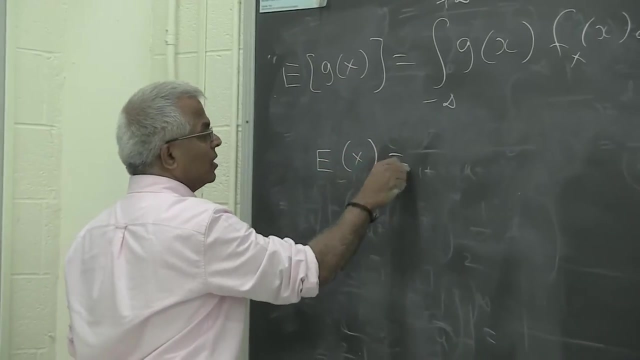 0. at this point this goes away. all these terms goes away except this. so we can extract the mean from here. So the mean is: you take the derivative, You take the derivative once and plug in omega equal to 0, so you get expected value of x. 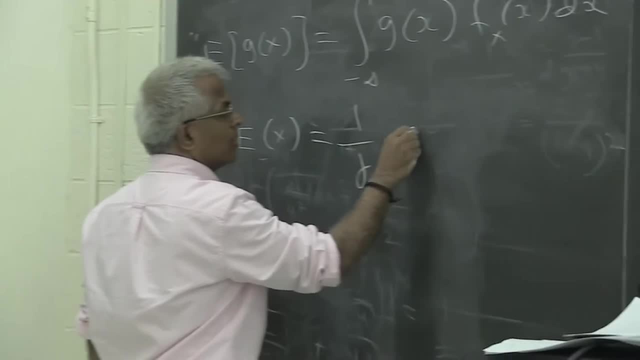 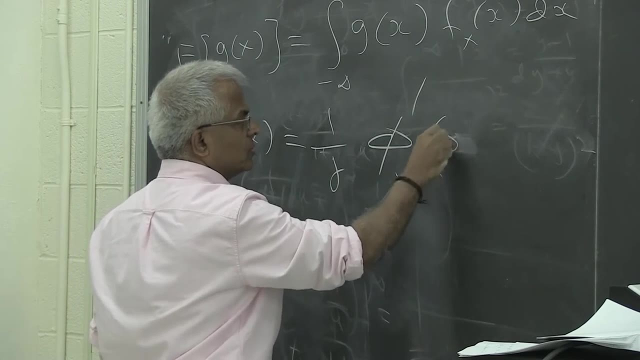 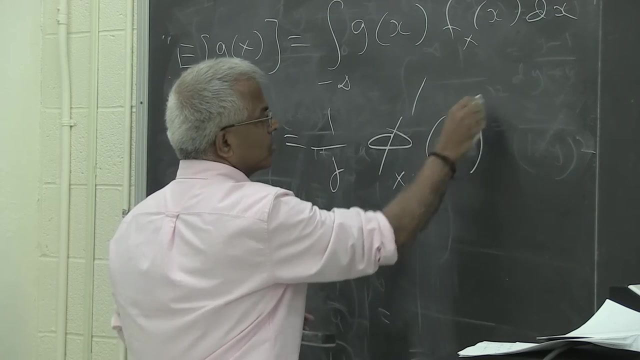 and then you have a j here, so I take the j to the other side. so the derivative of the characteristic function evaluated at 0, you can also write this as in this manner: at omega equal to 0. Now we would first do the derivative. 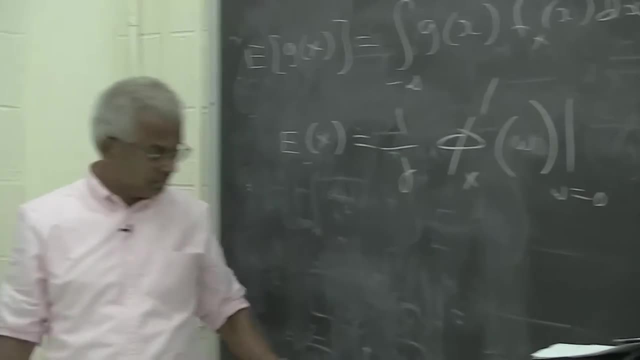 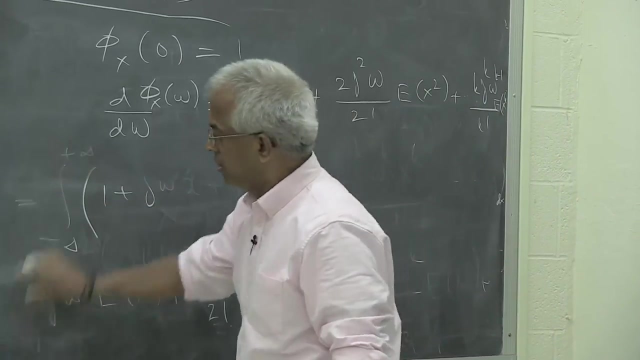 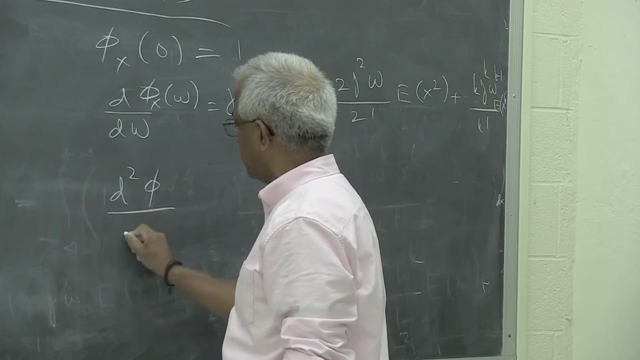 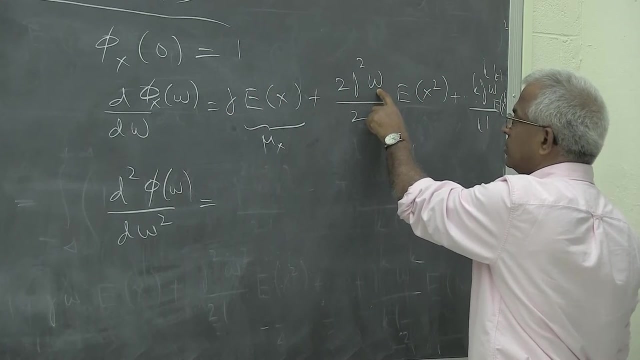 And then plug in omega equal to 0, now notice that what happens if you take the derivative one more time here, if you take a second derivative, this comes d squared d omega squared of this, so this is a constant- goes away. this is just omega, so the derivative is this constant. 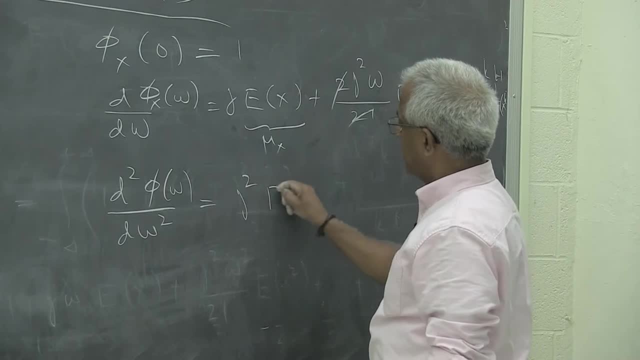 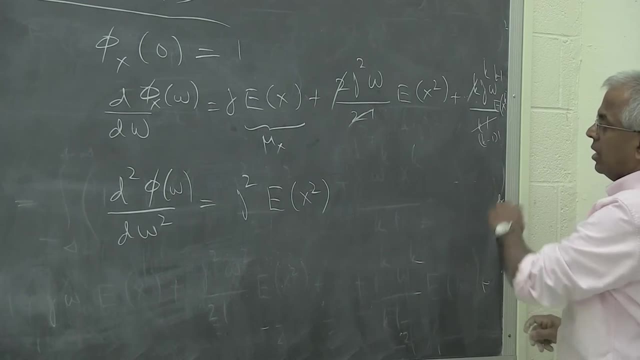 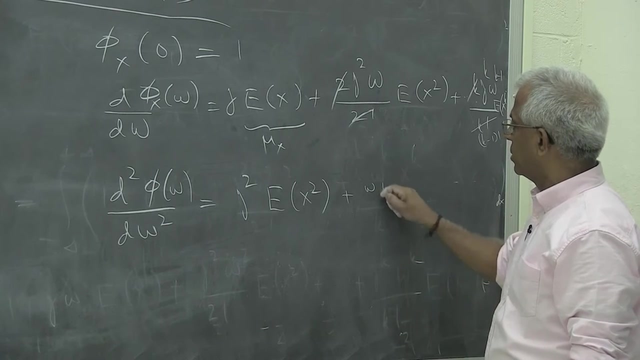 but this 2 and 2 cancels. So you get j squared expected value of x squared. here. this k cancels. you get k minus 1 factorial and the next term is going to be, of course, it's omega multiplied by x. 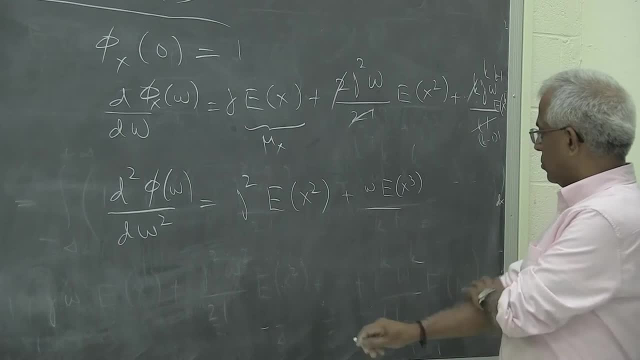 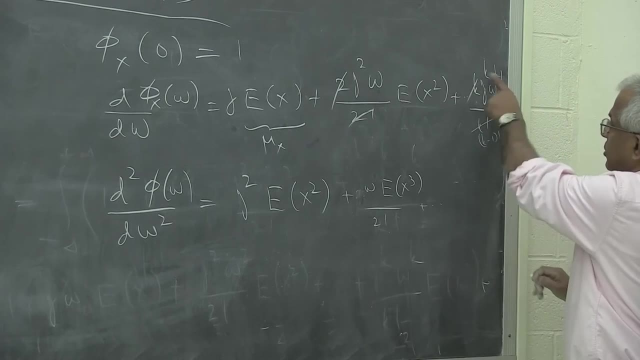 cubed, I think over 2 factorial previously, so plus, etc. you need to take the derivative of this one more time: q, k multiplied by k minus 1, again, k minus 1 cancels. so you have j to the power, k omega. 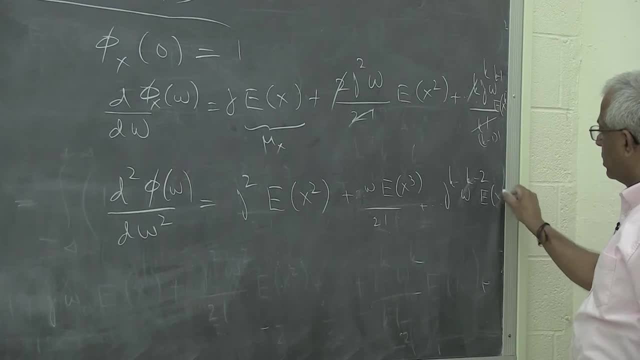 to the power k minus 2, now e, to the power xk over k minus 2, factorial, etc. because k cancelled, k minus 1 would cancel, so you would get k minus 2.. Once again the same stunt. if you put omega equal to 0, all these terms vanish, you get. 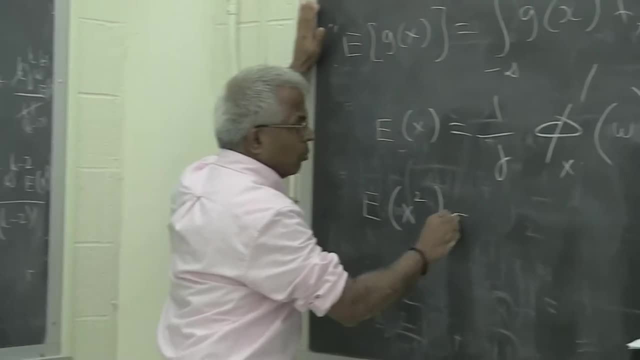 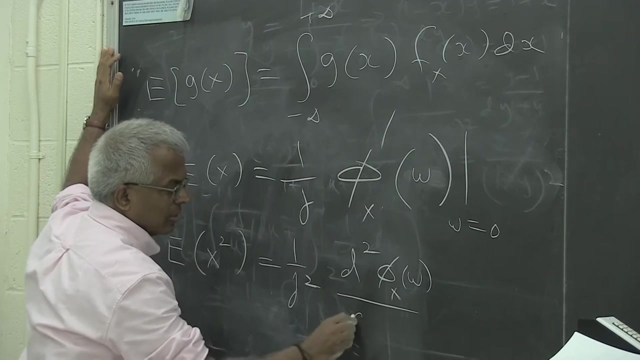 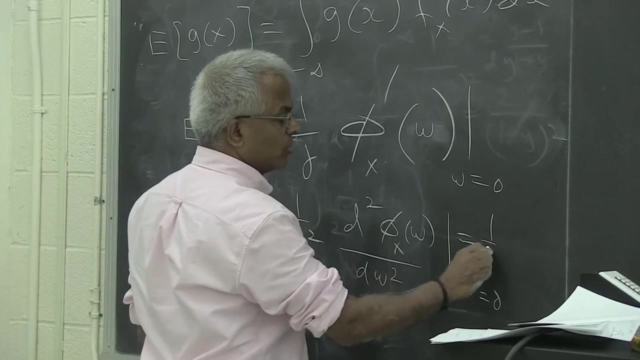 the second moment. so the second moment is going to be 1 over j squared, the second derivative of the characteristic function, and then you substitute omega equal to 0, so, if you are not confused, you can also write this as phi x 0, double prime. this is the second derivative. 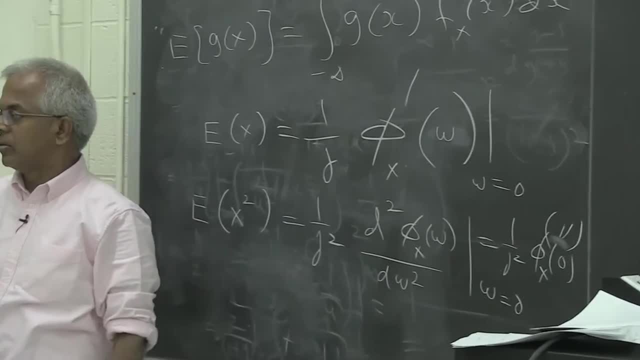 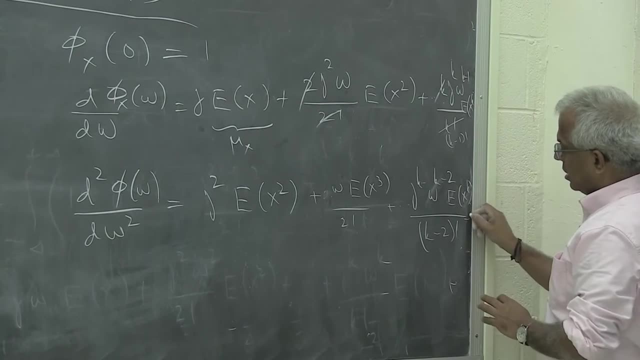 but we need to do the derivative first and then plug in omega equal to 0, you can see, you can continue this If you take this derivative. you can see, you can continue this. if you take this derivative k times, this will turn out to be a constant. and then if you substitute omega equal to 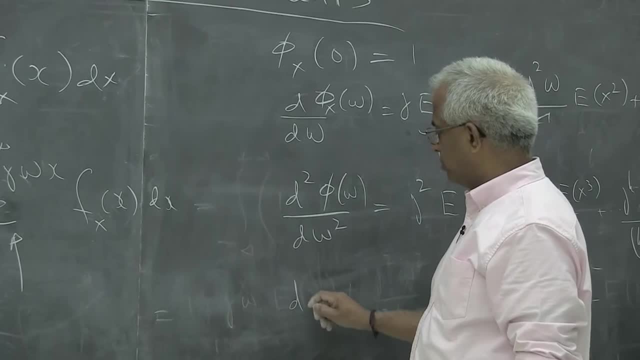 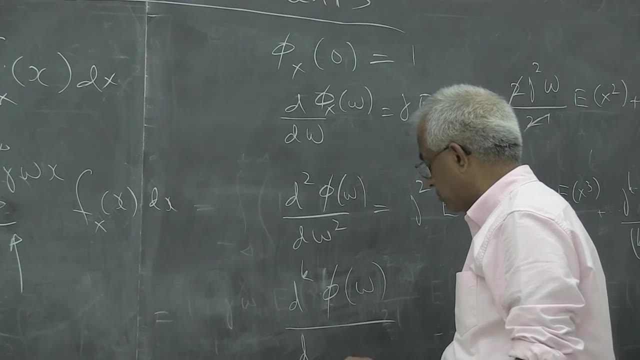 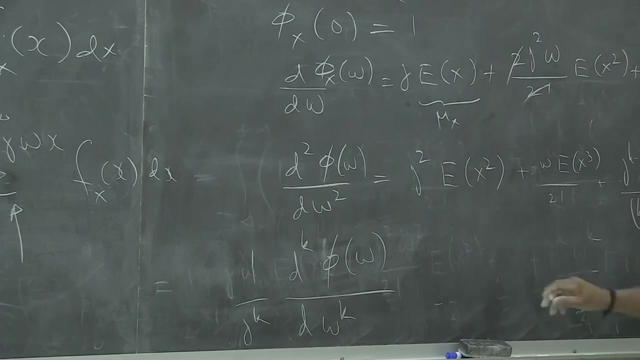 0, all the other terms will vanish. so if you take the derivative of this characteristic function k times and divide by 1 over j to the power k, you bring that there- then you can extract this by substituting omega equal to 0, you get expected. 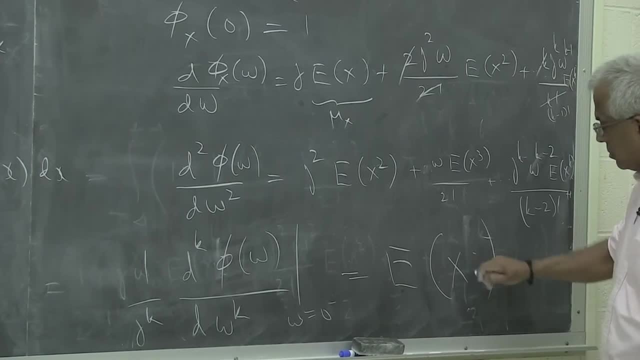 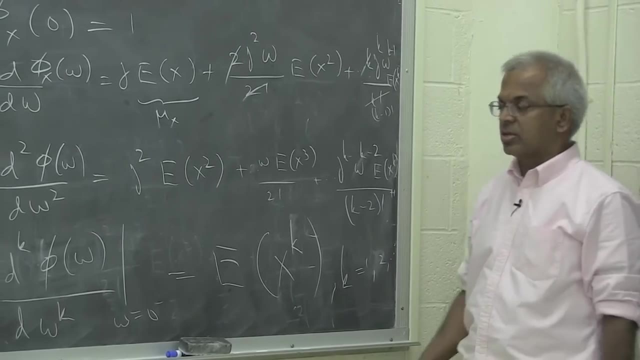 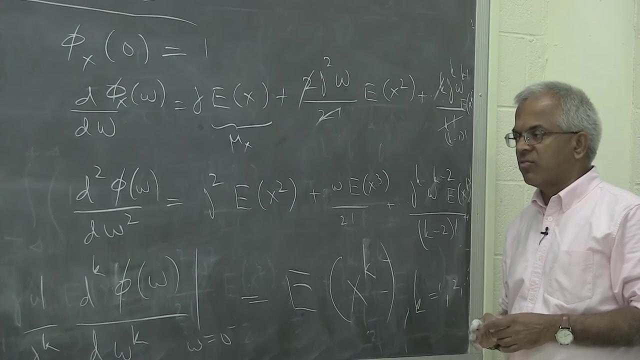 The expected value of x to the power k. So this is a useful formula to find all the moments for k equal to 1,, 2,, 3,, etc. So I will use this to derive the mean and variance of few random variables. 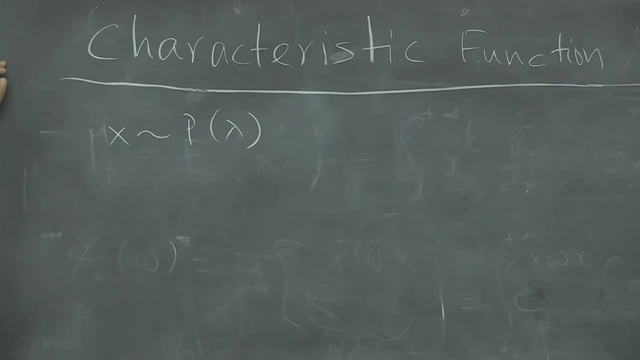 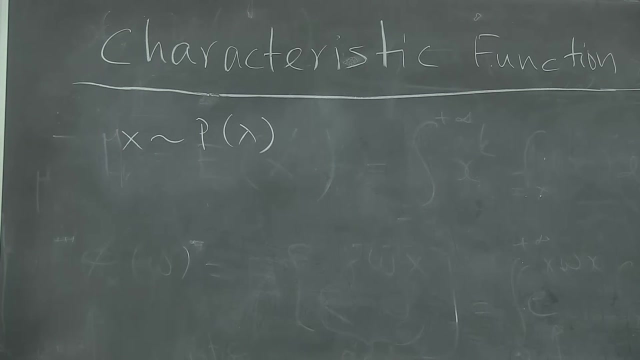 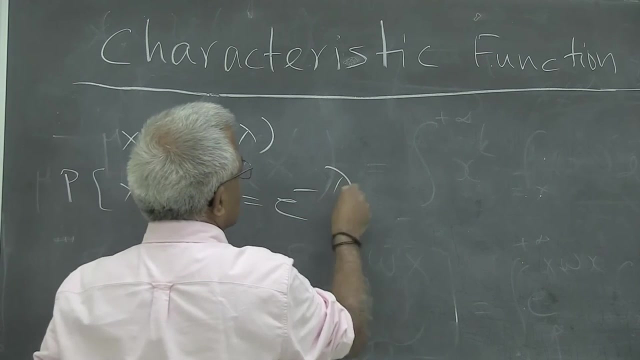 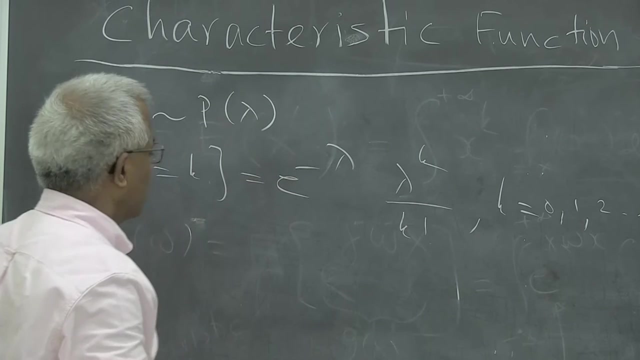 So let me illustrate the characteristic function: usefulness to compute the moments through few random variables. So we will start with the Poisson random variables. so what we mean is probability of x equal to k. is e raised to minus lambda, lambda k over k, factorial k equal to 0,, 1,, 2,, 3, etc. 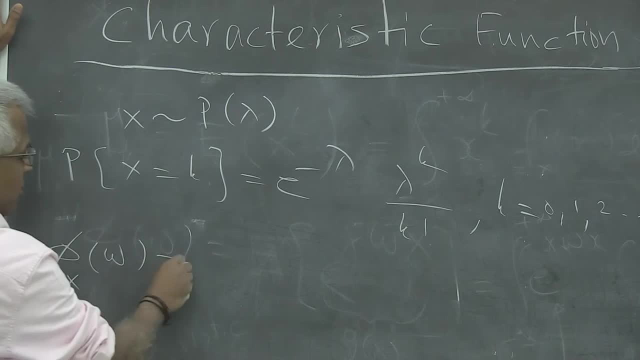 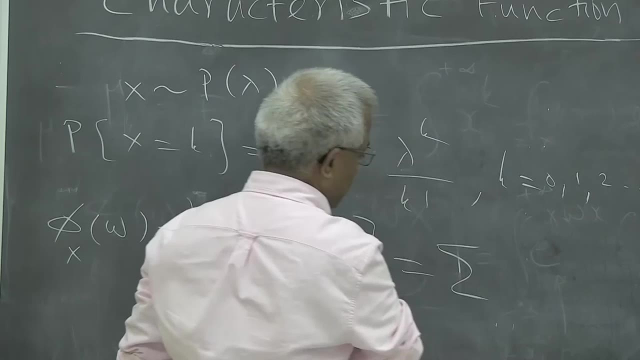 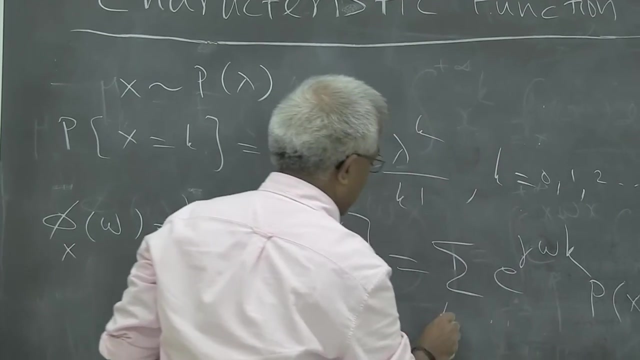 So let us find the characteristic function first. so characteristic function is expected value of e raised to j omega x. so this would be, so the function multiplied by which is e raised to j omega k, a probability of x equal to k right k goes from 0 through infinity. 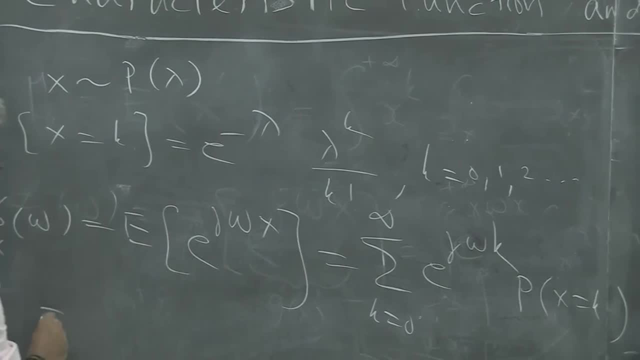 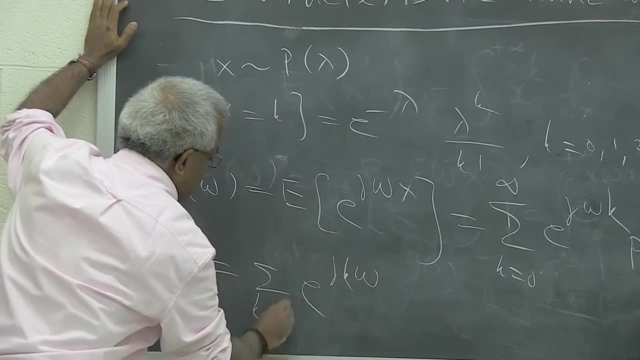 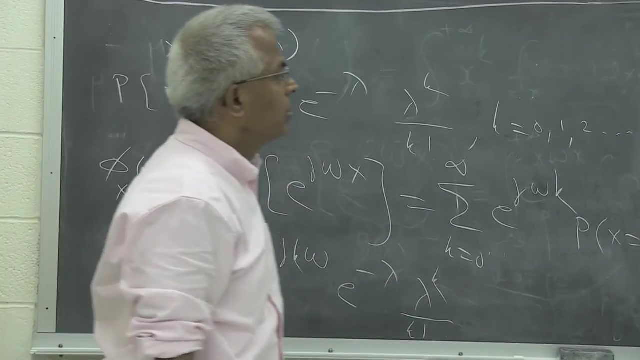 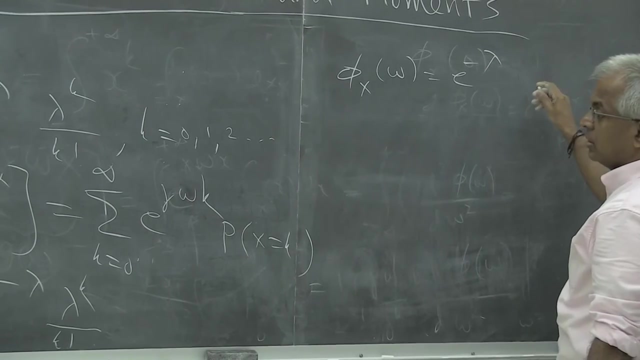 from here. So if I plug this in, this is summation: e raised to j k. omega k goes from 0 through infinity. e raised to minus lambda, lambda k over k, factorial. so rewriting it here: characteristic function of x is: So if e raised to minus lambda goes outside, then the rest seems to be lambda e raised. 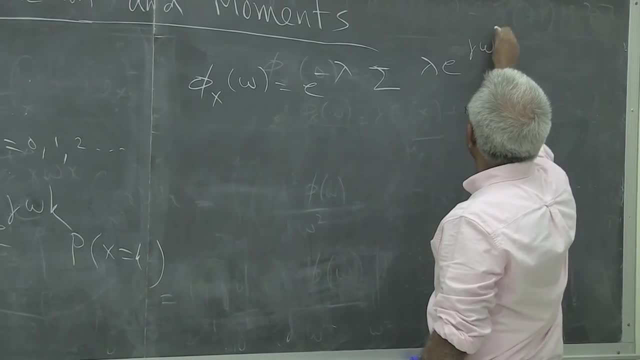 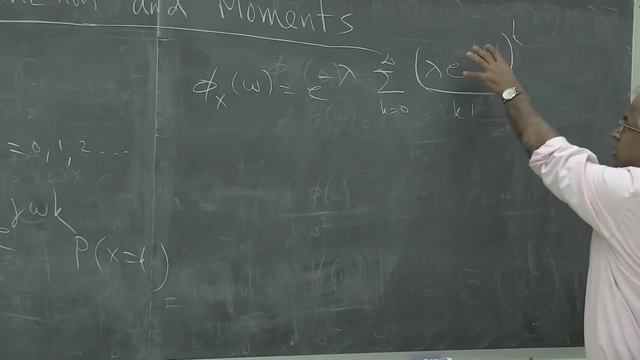 to j, k, j, omega, whole thing to the power k over k factorial. k goes from 0 through infinity. Notice, this is of the form something, z to the power k over k factorial. so this is the expansion of e raised to z. in other words, the characteristic function turns out to be: 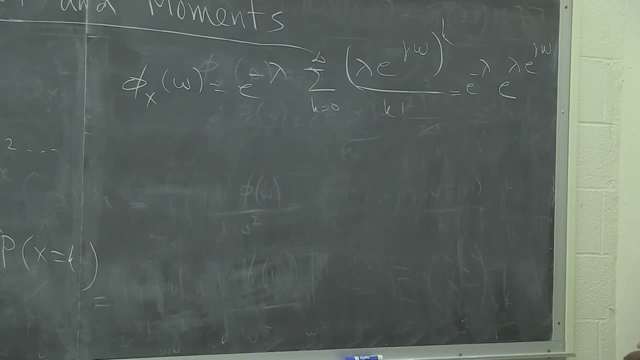 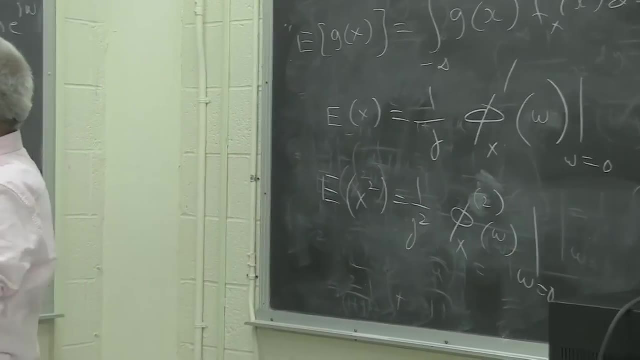 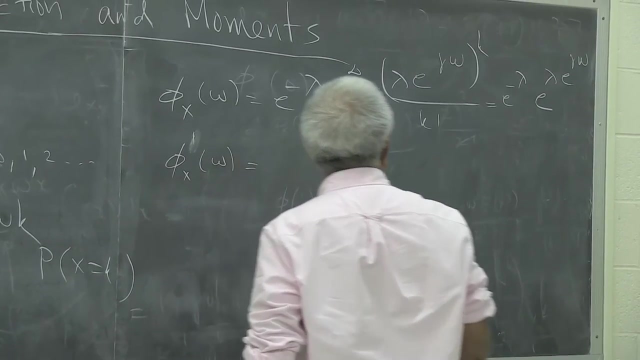 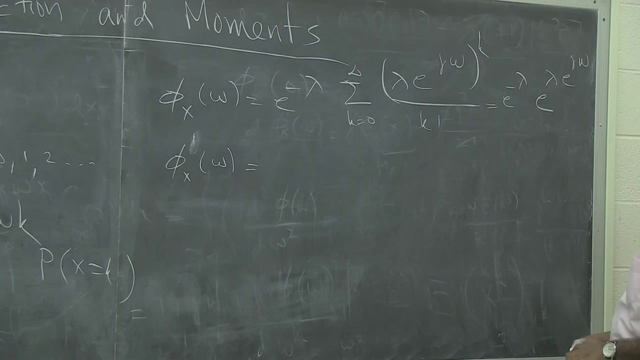 this is the characteristic function of Poisson random variable. Now we can use this formula to find its mean. So we take the derivative of this with respect to omega first once. so the derivative is going to be So: notice, I can this. if you want, I am going to combine. 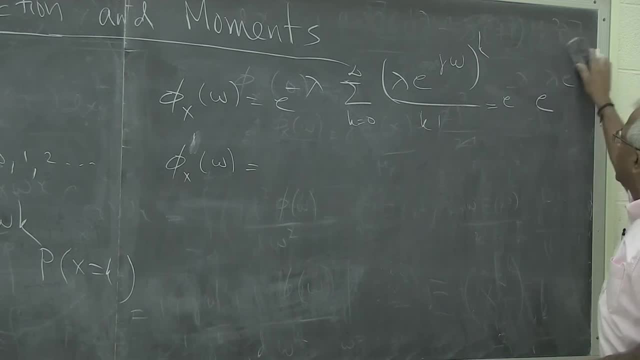 Okay, right, Right, This is perfect. At least you have got a Concept together. so this is e raise to minus lambda, 1 minus e raise to j omega. it's combining the two. previously we had e raise to minus lambda multiplied by e raise to plus lambda. 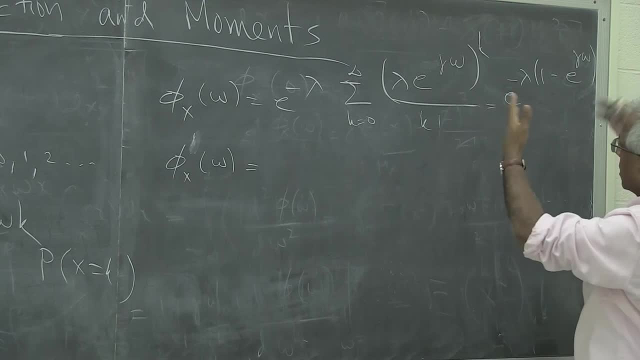 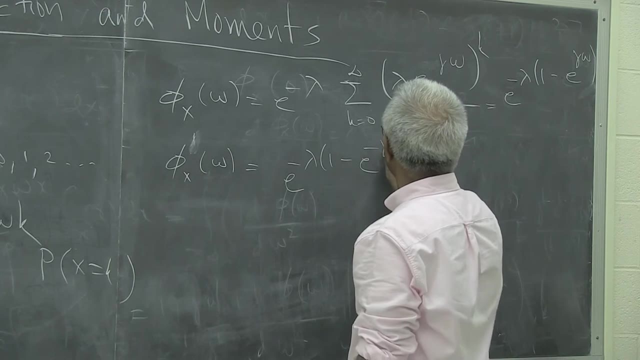 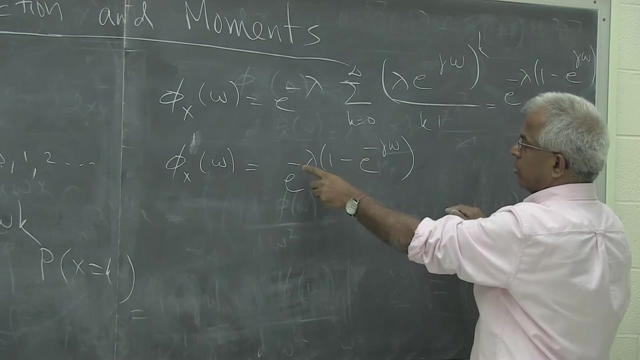 j omega. so remember, the derivative of e to the power is itself. so e raise to minus lambda, 1 minus e raise to minus j omega, then multiplied by the derivative of this with respect to omega, so that's going to be multiplied by lambda from here. remember this is a constant. 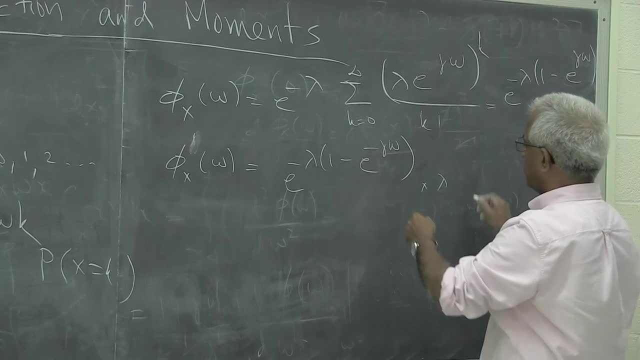 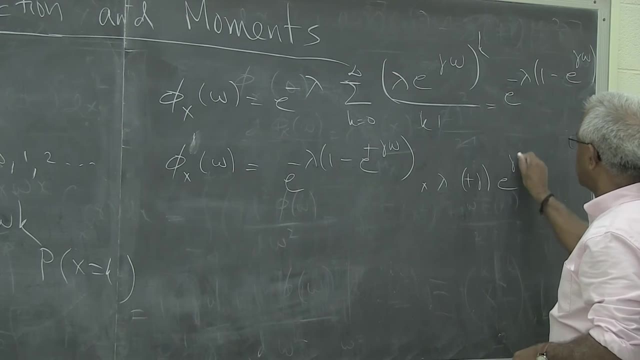 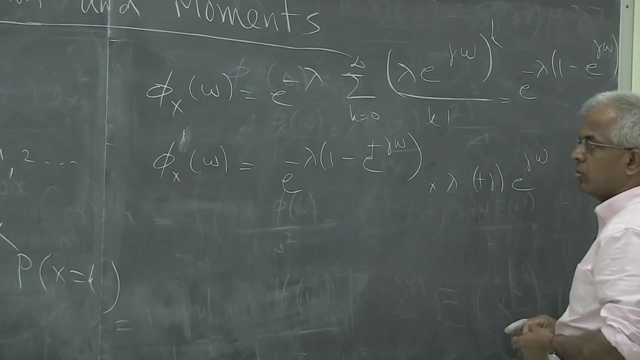 so minus, minus, plus lambda. then the derivative of this, which is minus, this is plus here, so that's going to be plus. j e raise to j omega. this is the derivative. so now we put omega equal to 0, omega equal to 0, this is 1, 1 minus 0. 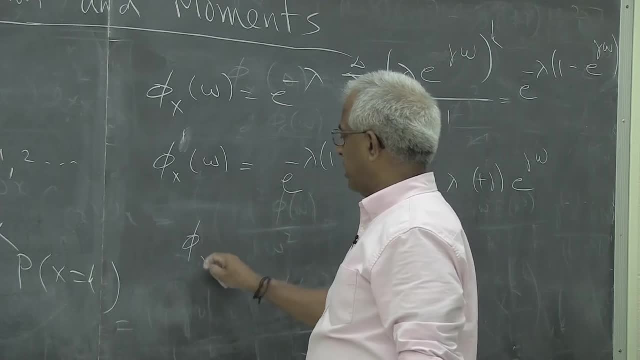 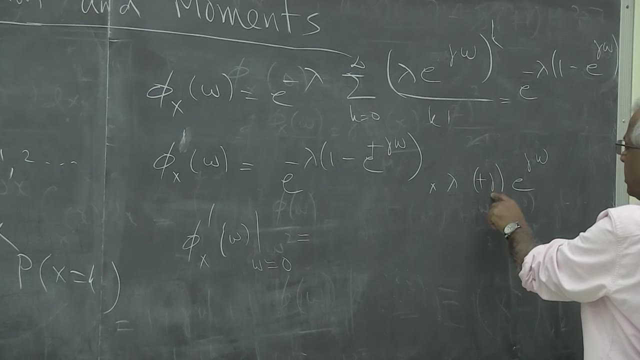 e raise to 0 is 1, so phi x sub prime omega at omega equal to 0, so this is 1, this is lambda. this is j. this is omega equal to 0,. this is 1, so the answer is j, lambda. so 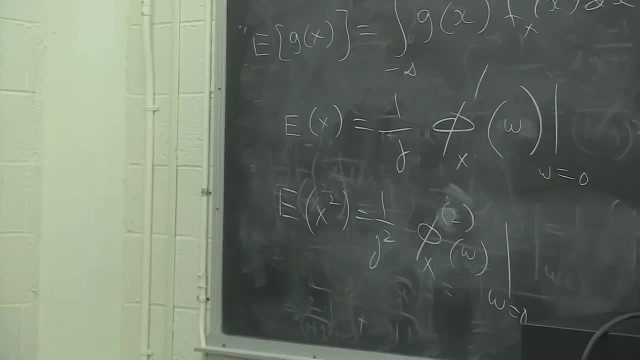 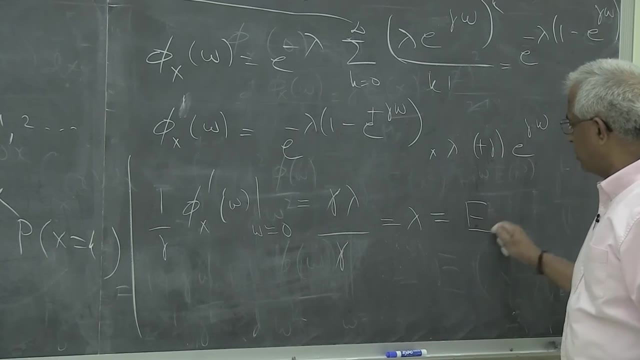 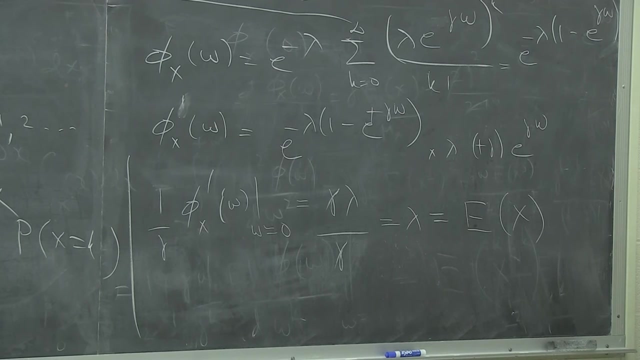 to get the first moment. we divide by j, so we divide by j, so that j, j cancels. so you get lambda to be the first moment. so that's the mean of the Poisson reaction. So if you want to compute the variance, we need the second moment. so let me just do. 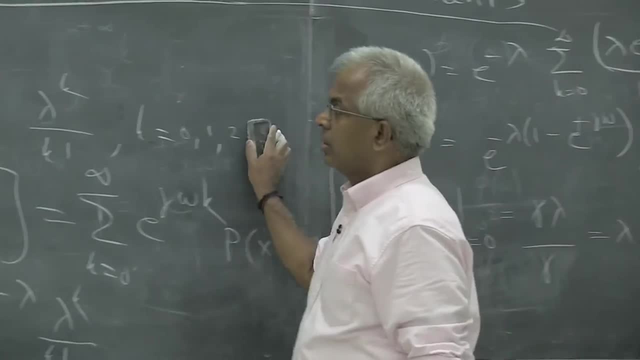 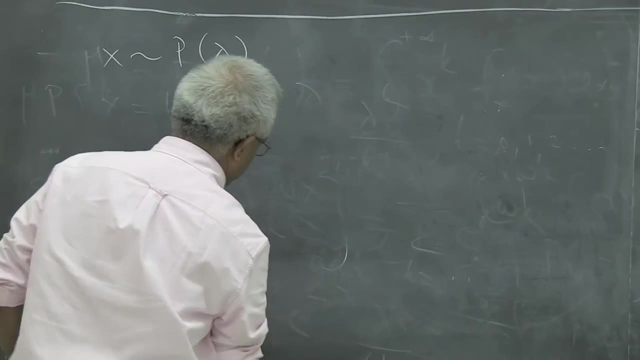 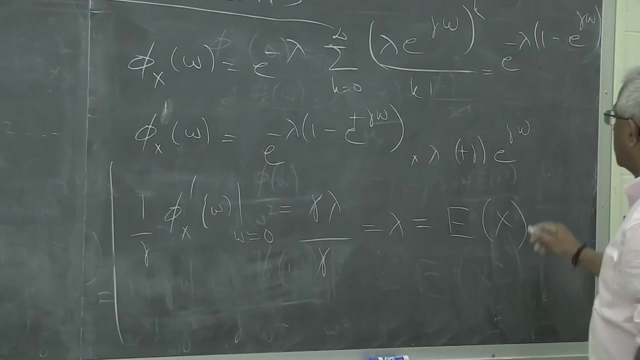 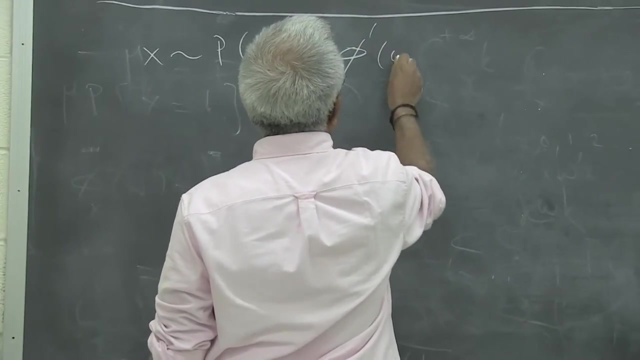 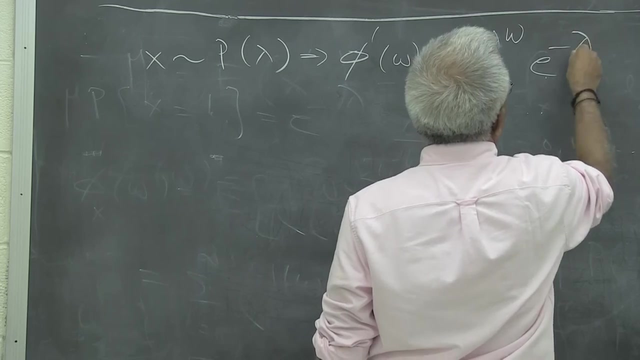 that quickly. here we already have the first moment, so all we need to do is take the derivative of this function. the first derivative is already here, so this is- I will rewrite it here- the first derivative to be lambda: e raised to j omega, then e raised to minus, lambda 1. 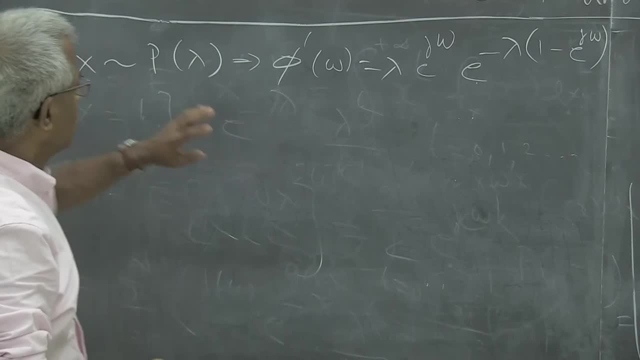 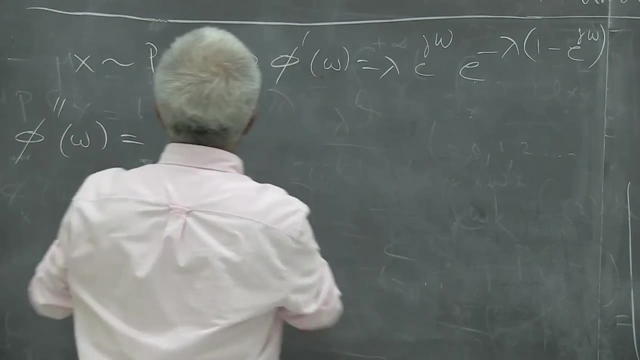 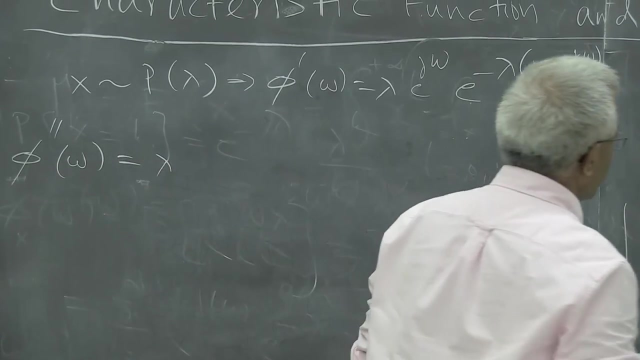 minus e raised to j omega, so we can do this by parts. the second derivative: remember the derivative is with respect to omega, so lambda is a constant. so first the derivative of this, which is just multiplied by a j. there is a j here, so j lambda is a constant. then the derivative. 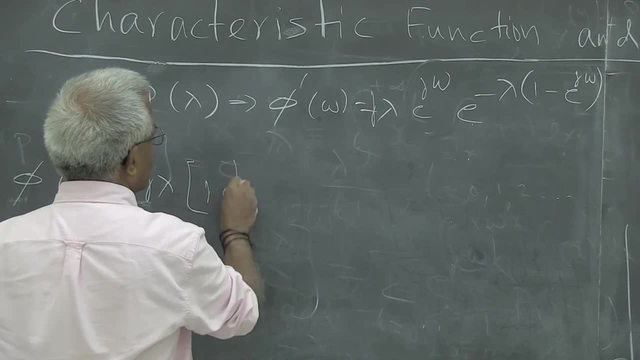 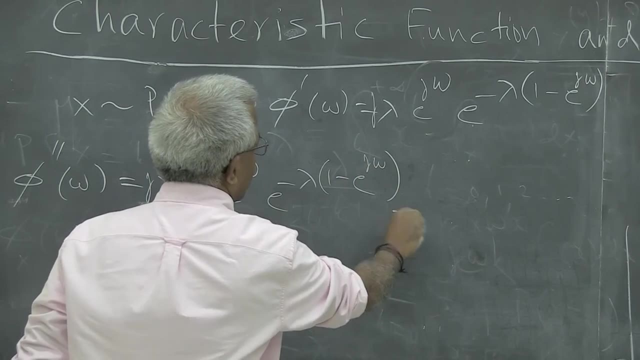 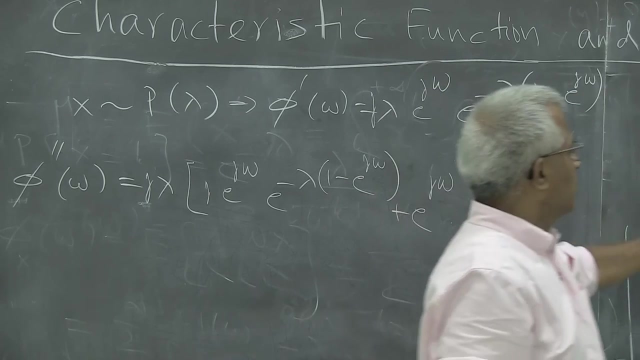 of this, which is just j e raised to j omega, then the second function as it is, then the second function stays. this first function stays, the same e raised to j omega, derivative of this, which we already have it here. so I am just going to copy from here: 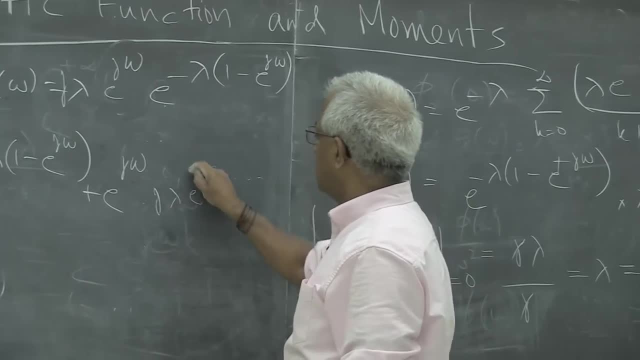 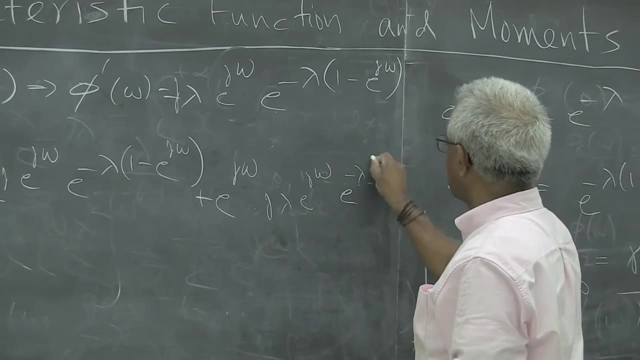 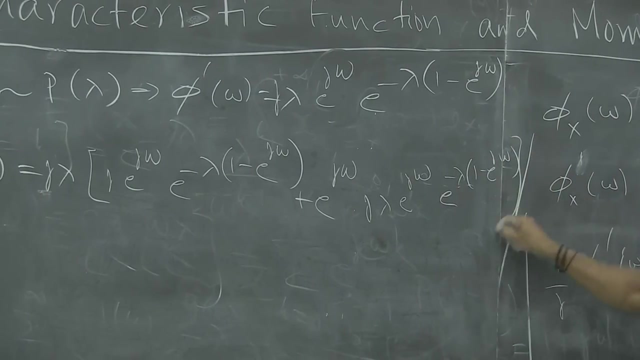 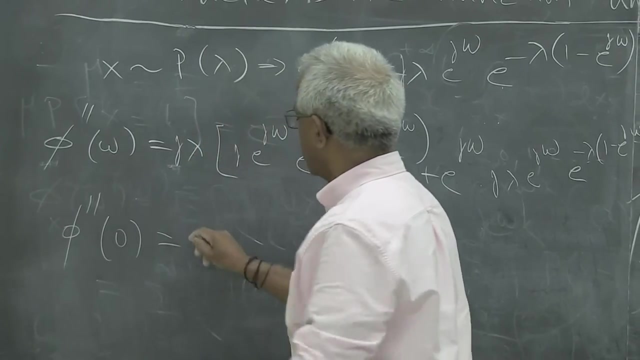 Okay, So the derivative is going to be j lambda, e raised to j lambda, e to the power minus lambda. or you can do it one more time. now you substitute omega equal to 0 at this stage, so you need to do this. so you have j lambda here. here you have a j, here you have a j, so this becomes j square. 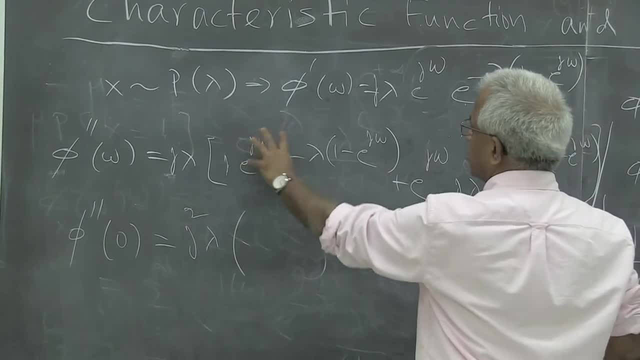 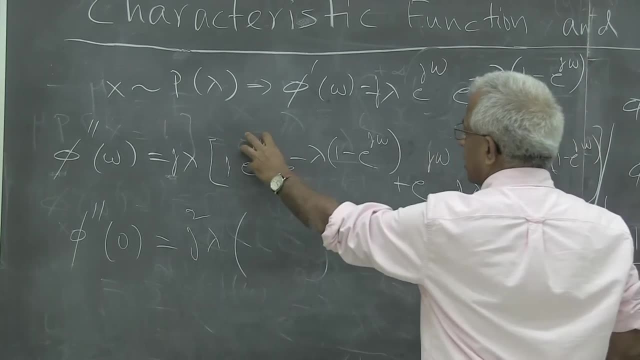 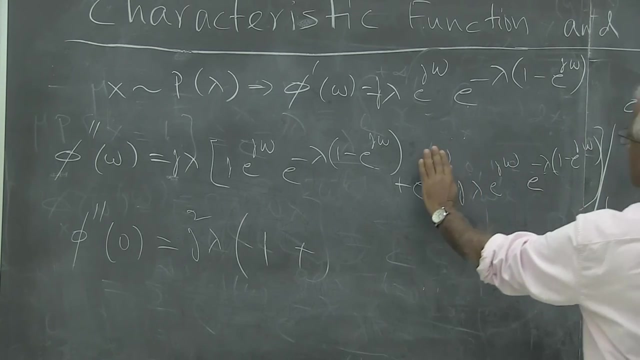 outside, and this is 1, this is 1,. when you put omega equal to 0,, this is 1, 1 minus 1, 0, so e to the power- 0 is 1,. omega equal to 0, this is 1, so this is simply 1 plus this is 1 here. 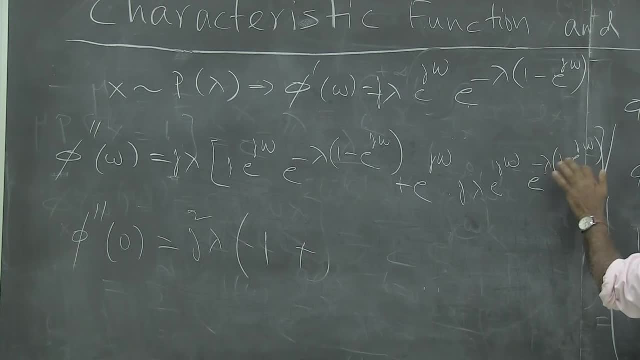 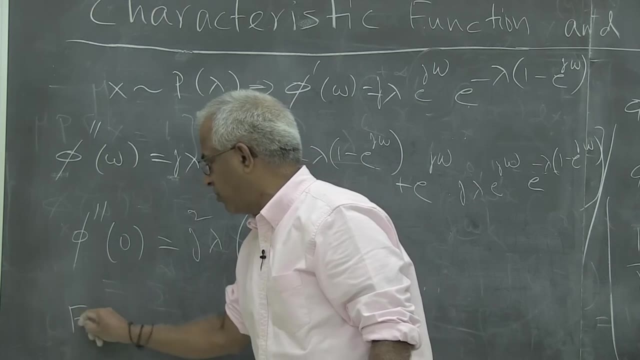 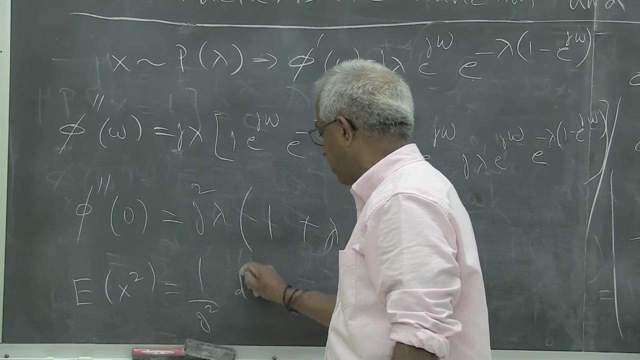 this is 1, this we just went through. this put omega equal to 0, 1 minus 1, 0, 1 plus lambda. so expected value of x squared is 1 over j squared multiplied by the second derivative of the characteristic function. 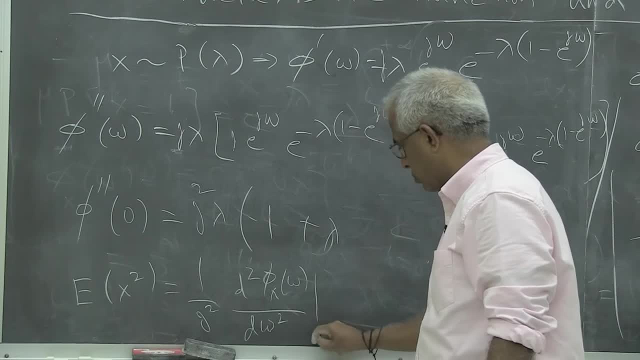 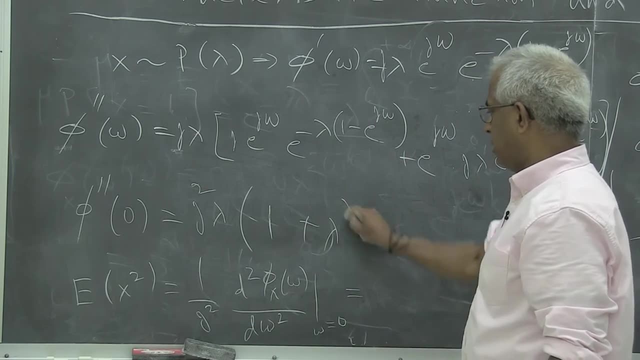 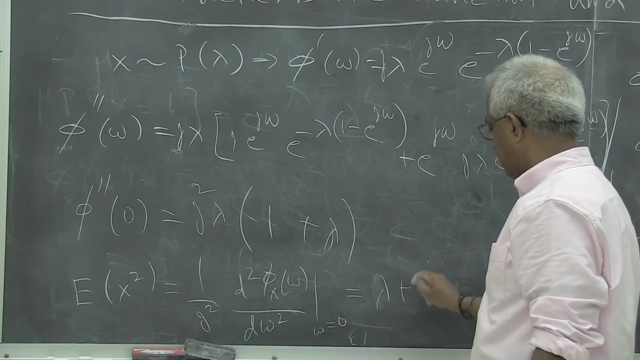 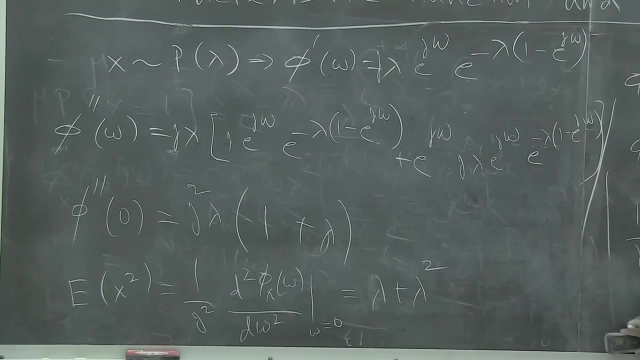 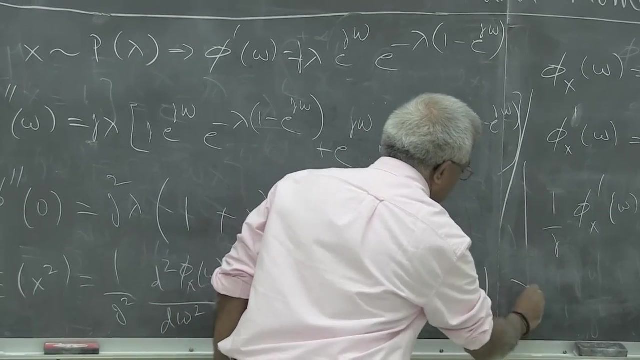 you put omega equal to 0, omega equal to 0, which we have here, so j squared cancels. so this turns out to be lambda multiplied by 1 plus lambda, which is lambda plus lambda squared. so, that being the case, we can now derive the variance. so this gives us the variance of the Poisson random variable. 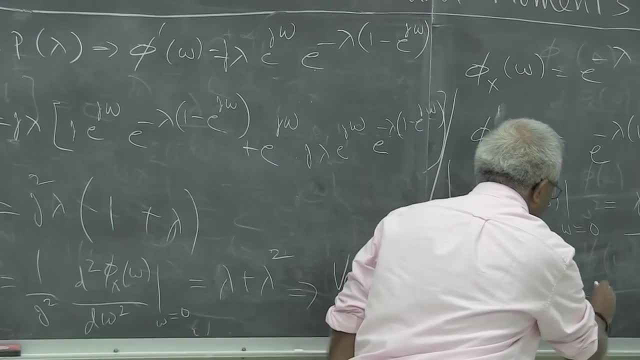 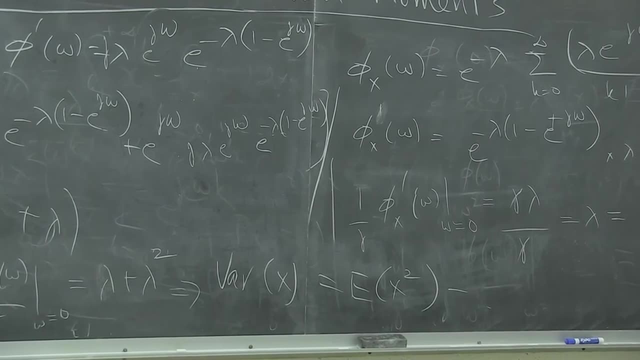 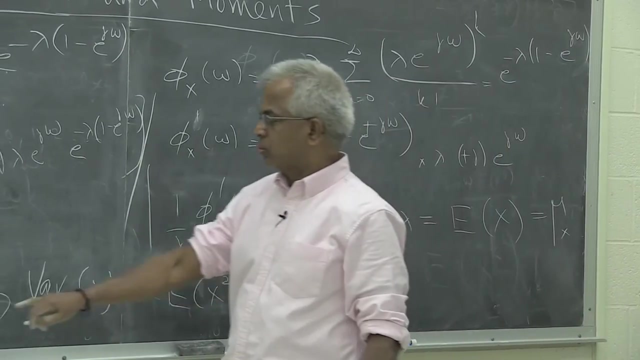 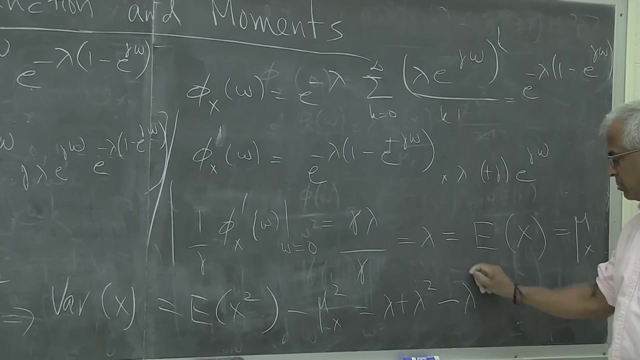 to be expected value of x squared minus its mean squared, which is here. the mean of x is here, minus mu x squared. but expected value of x squared is lambda plus lambda squared, so lambda plus lambda squared minus the mean is lambda, so that's lambda squared. 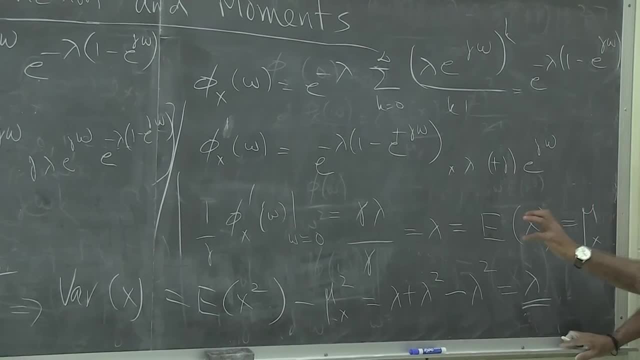 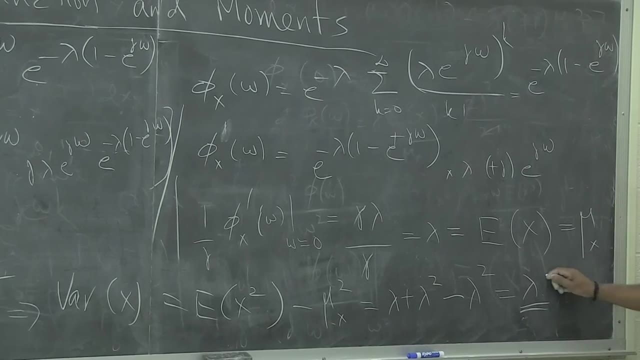 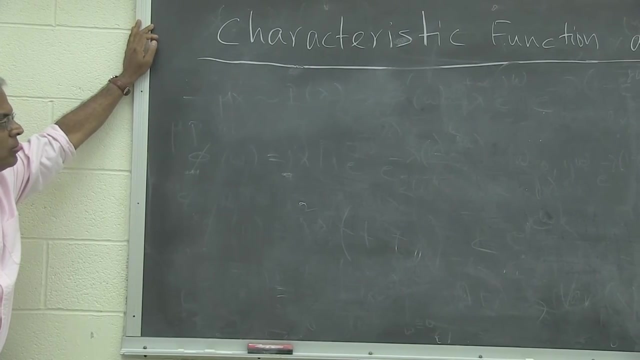 so this turns out to be lambda. so, interestingly for Poisson, the mean and variance are numerically the same: mean is lambda, variance is lambda. lambda is of course positive, so everything checks. Let's look at another example which, let's say, x is binomial with the mean, with the two parameters. 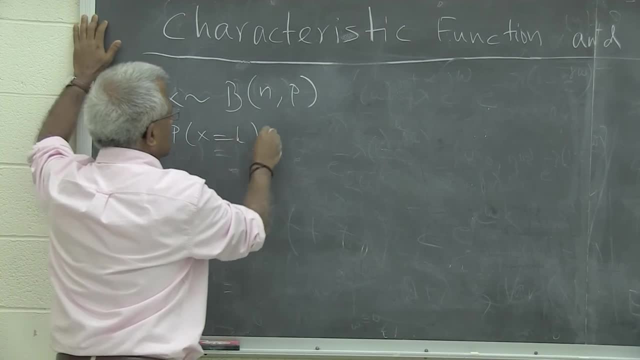 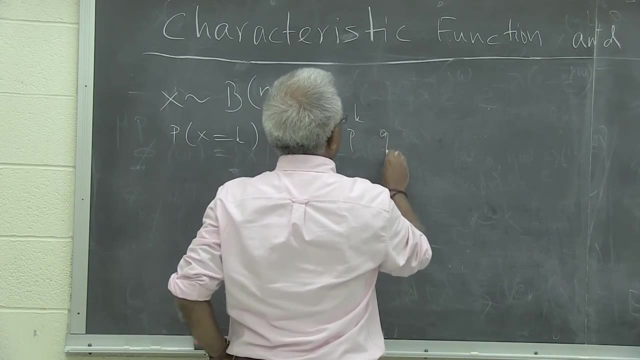 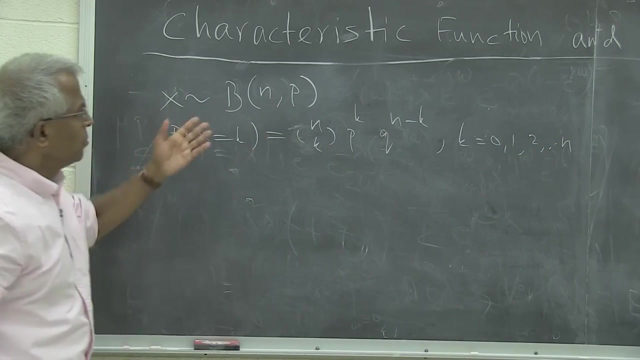 n and p, n and p. this means probability of x equal to k is n, choose k, p, k q to the power, n minus k, k equal to 0,, 1,, 2,, 3 up to n. so let's find the mean and variance using the characteristic. 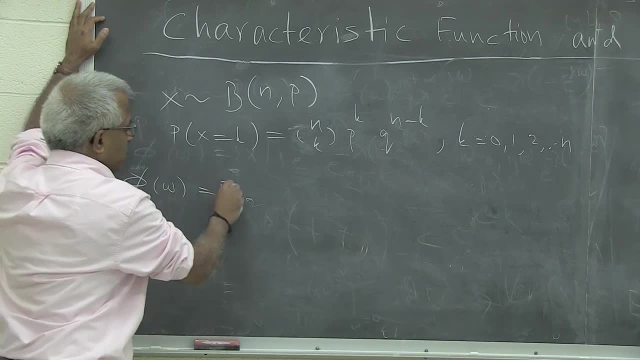 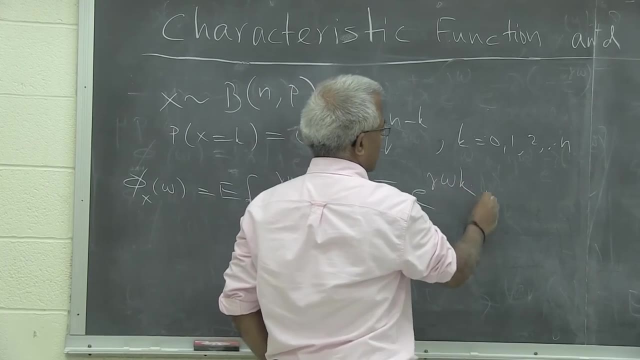 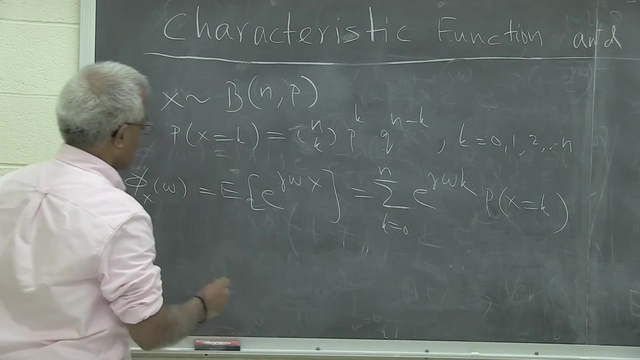 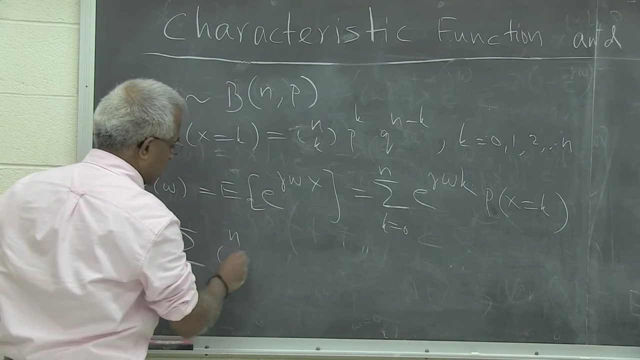 function. so first of all, characteristic function is expected. value of e raised to j omega x. this is summation: e raised to j omega k. probability of x equal to k. k goes from 0 through n. so if I substitute for probability of x equal to k here, this reads now: n, choose k. I have 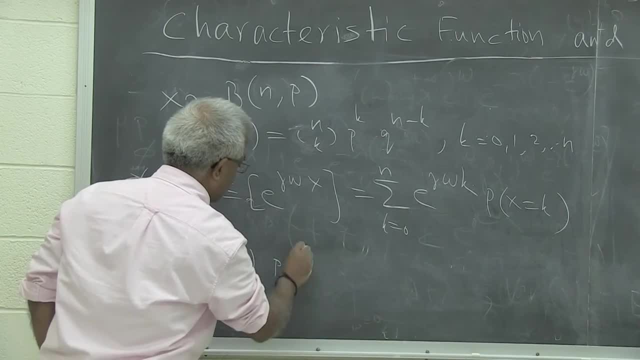 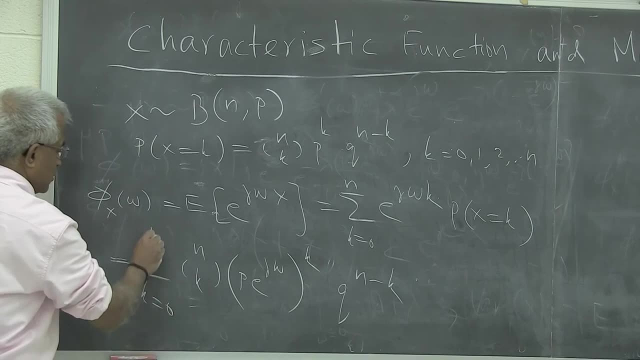 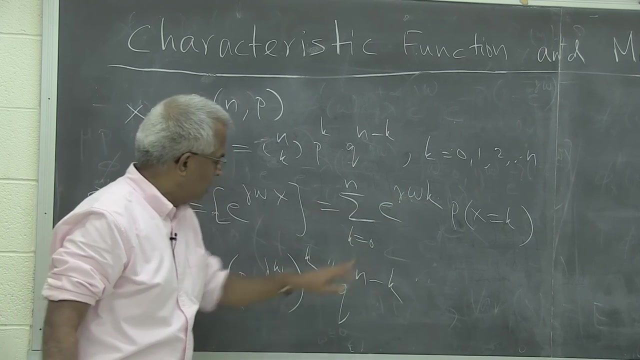 p to the power k, e to the power, j omega k. so I can write it together as in this fashion: so let's see what happens, What I have done, n choose k from here. I have p to the power k. I have e raised to j omega k. e raised. 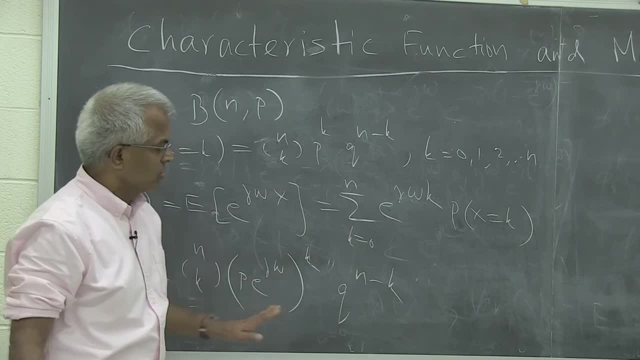 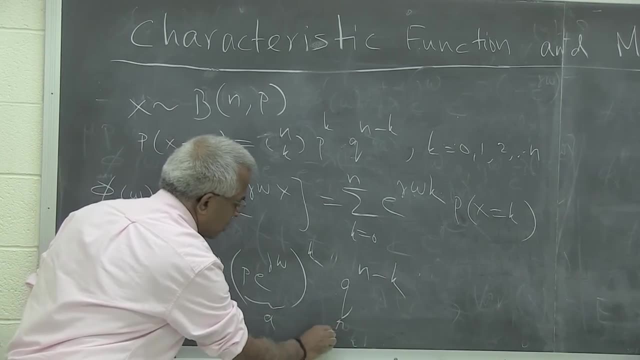 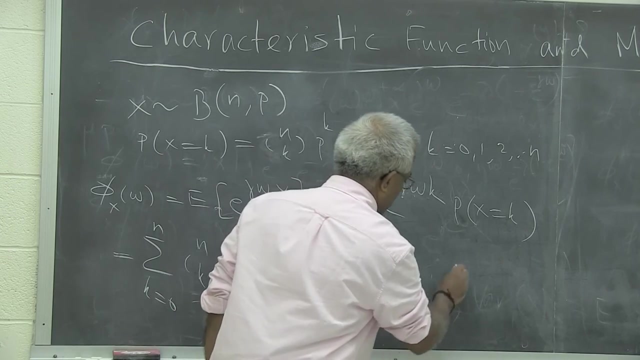 to j, omega k and q to the power, n minus k. so everything is. if you call this to be a and q to be b, this is the expansion of a plus b to the power, n n choose k, a to the power, k b to the power. in other words, this whole thing can be written as: where a is p, 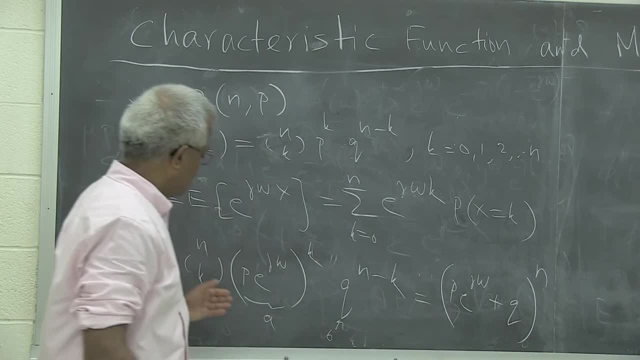 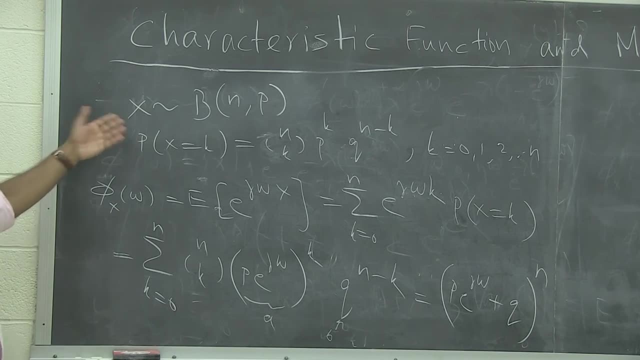 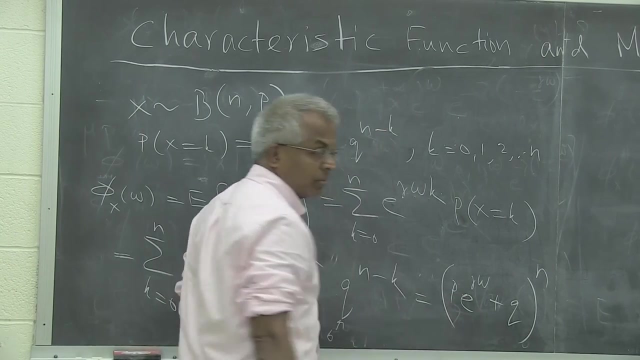 e raised to j omega And q to the power n minus q. you just have to identify this as binomial expansion. that's why we call this random variable to be binomial also. So this is the characteristic function of e raised to j omega k. this is the characteristic 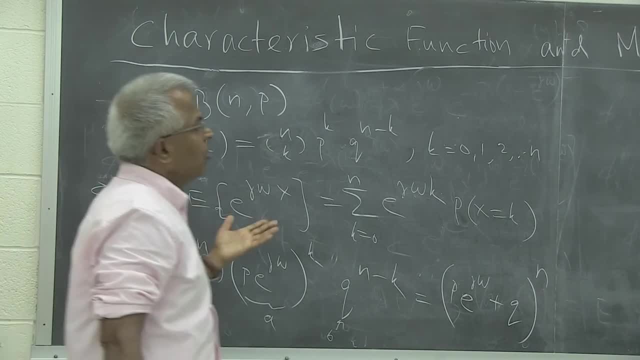 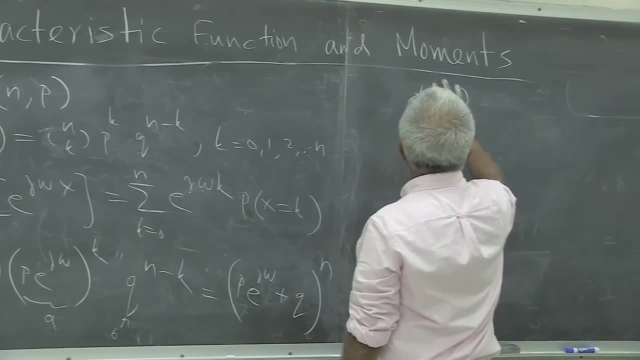 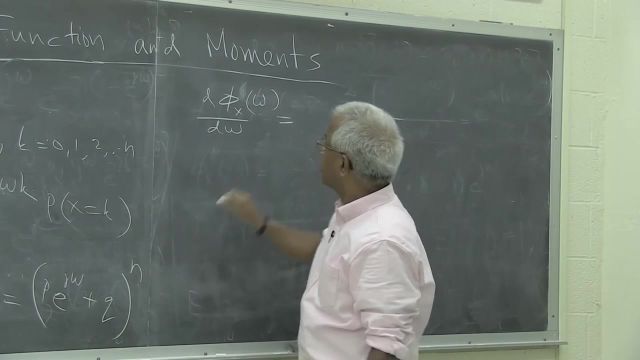 function of binomial random variable. so now we can, once we have the characteristic function, we can find its a first function. So now we can, once we have the characteristic function, we can find its a first function: derivative. and the second derivative, remember, derivative is with respect to omega. so this: 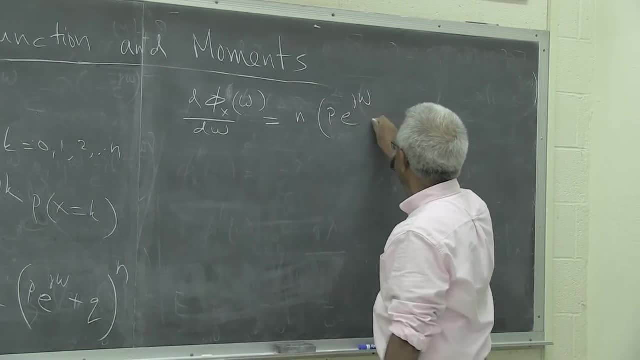 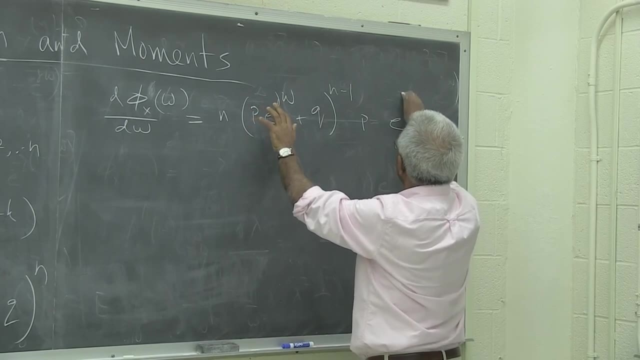 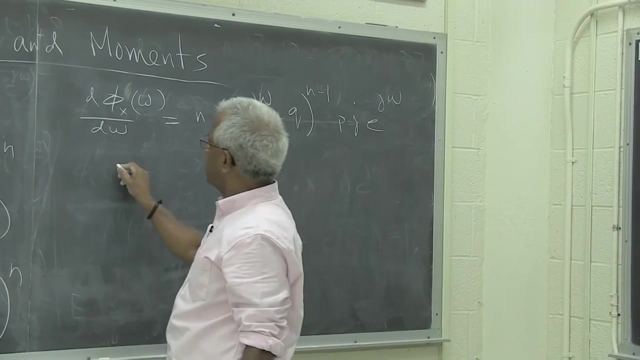 is n multiplied by p, e raise to j omega, plus q to the power, n minus 1 multiplied by the derivative of this, which is j, p, e raise to j omega and j. So now we put, if you put so, this derivative here, if you put so, this is d Phi omega over. 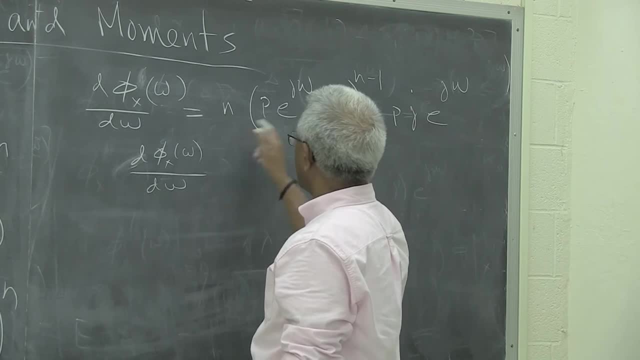 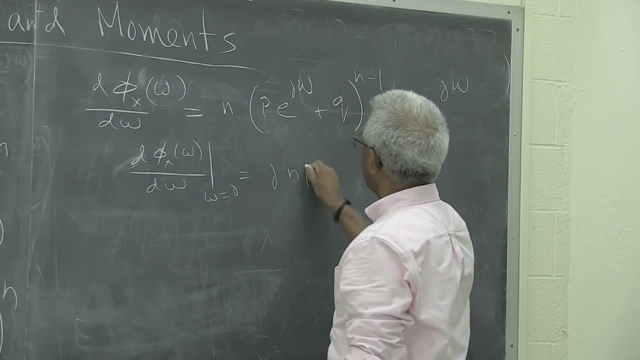 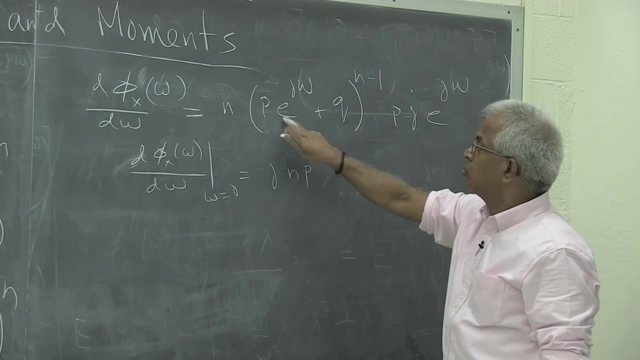 D, omega. if you put omega equal to zero, now what is that? also, you have j and p. n is here, p is here, j is here, omega equal to zero. this is one, omega equal to zero. this is one, p plus q is one. so one to the power. 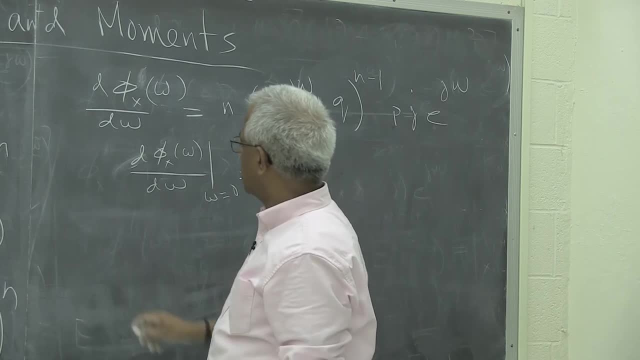 So So you get n like this: zero with 0 plus 1, D, omega equal to 0, omega equal to 0. this is get this answer. so if you divide this by J, J goes away and that's going to be NP. 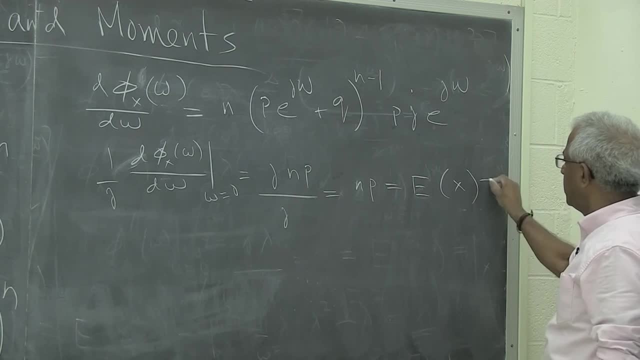 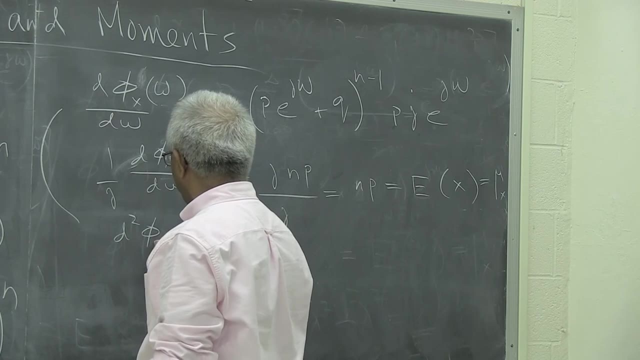 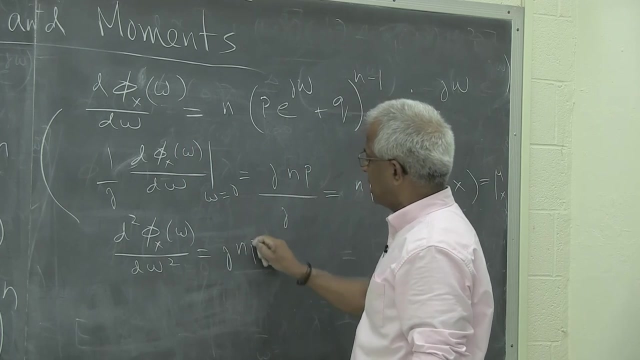 and that's your mean by definition. so we got the mean. so let's to find the second moment. we take the derivative of this one more time: d square, d phi omega over d omega square. first of all, let's the constants of J: NP is a constant, then you have two terms. 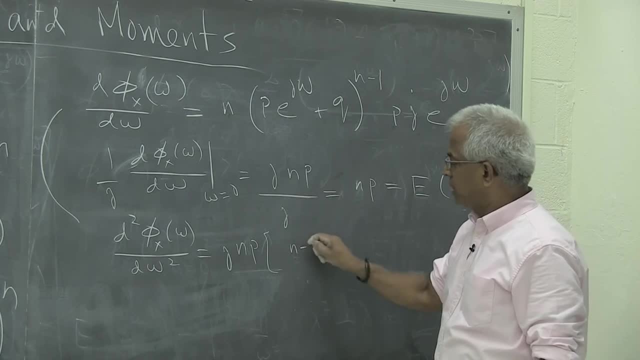 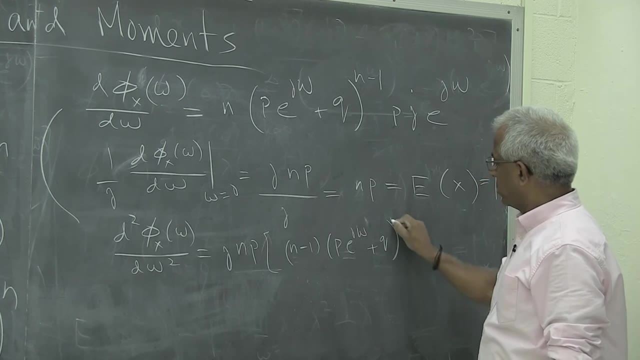 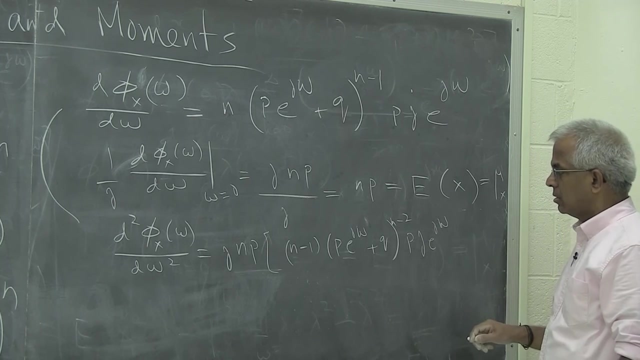 so let's just do it by parts. so this is first part. is N-1, p, e raise to j, omega plus q to the power N-2, multiplied by the derivative of this, which is p, j, e raise to j, omega plus, the first part stays the same- and multiplied by the derivative of this quantity, which is: 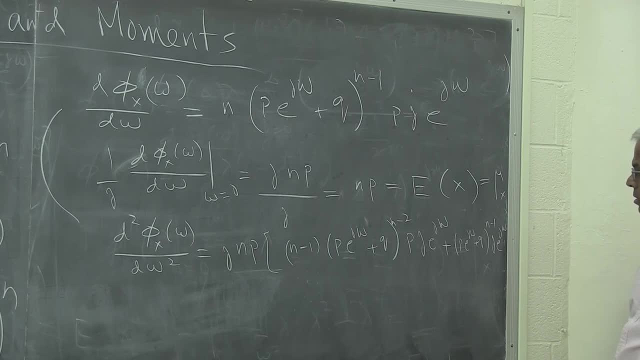 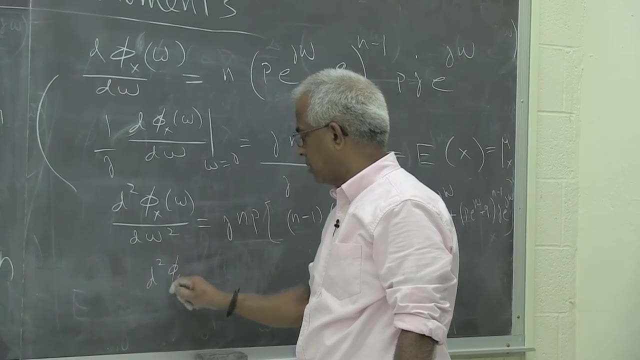 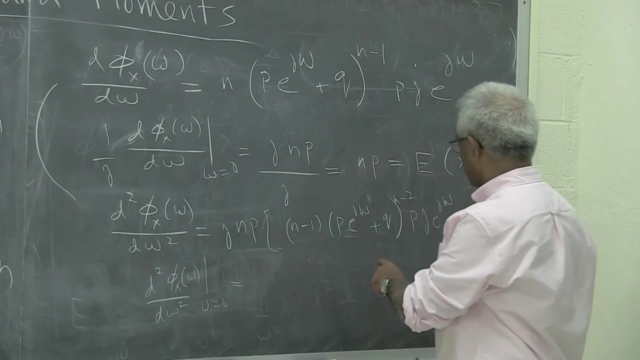 simply j e raise to j omega. All right, now we can substitute omega equal to 0, so when we evaluate the second derivative at omega equal to 0,, what is that? there is a j here. there is a j here, so J square goes. 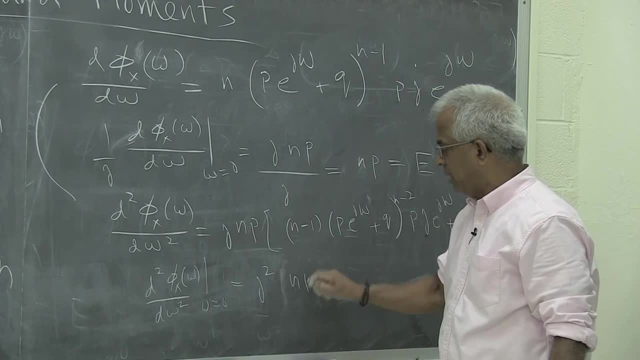 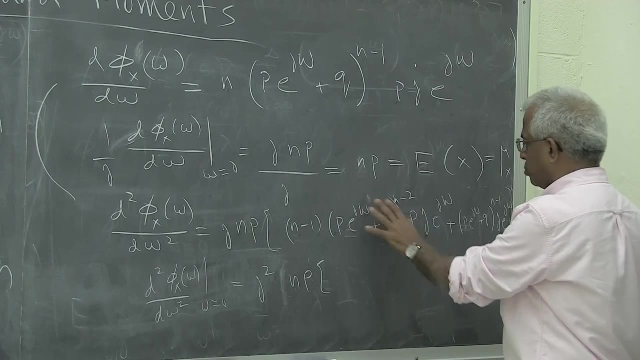 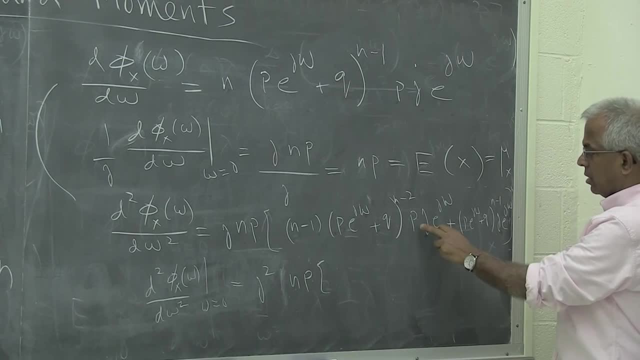 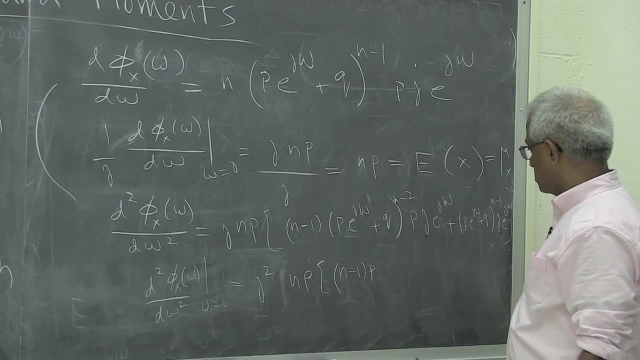 This is 1.. So from here you have 1, here you have p, N-1, p plus 1, I guess which, if you want, we can write as j square. So this is 1.. This is 1..